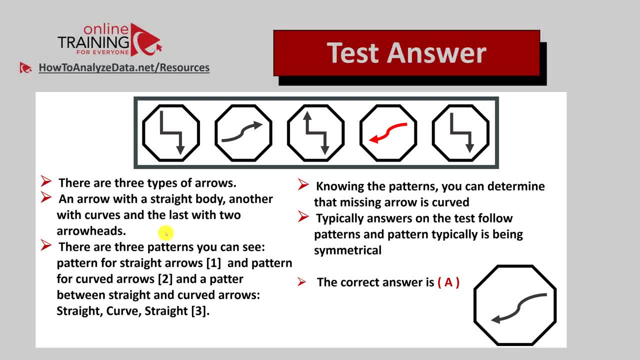 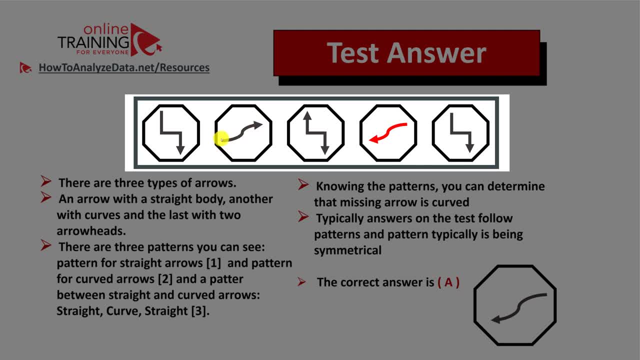 As usual, my recommendation is always: look for patterns. You see that the numbers one, three and five are straight arrows, And then we have a pattern for curved arrows. You see that the shape two and four contain curved arrows, And then you also see that the pattern of straight arrows. 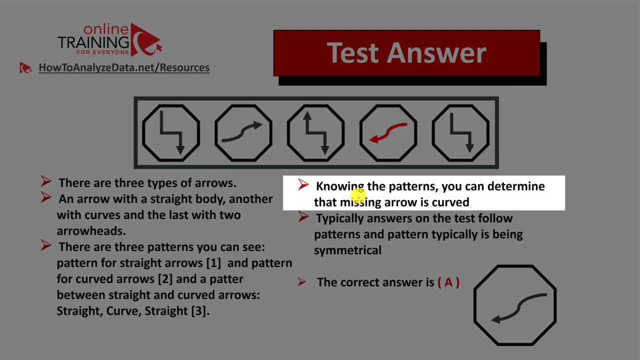 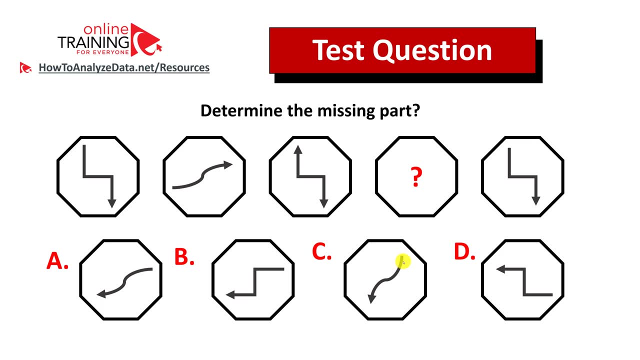 going down in the first and in the fifth shape. Now, knowing the patterns, you can determine that the missing arrow is curved. but as you can see, there are at least two curved arrows. And to typically the patterns on the test is symmetricity. so the arrow in choice C is not symmetrical to. 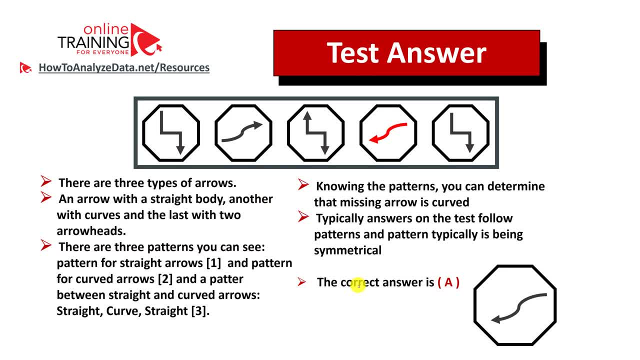 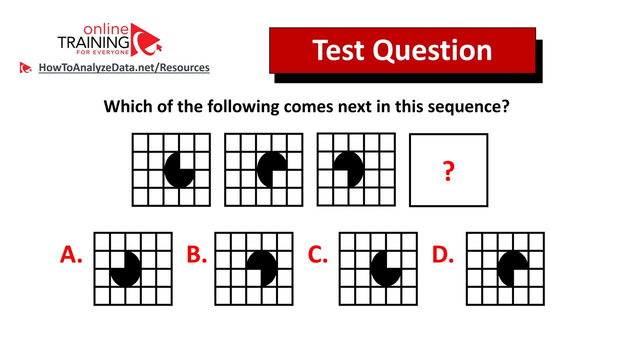 the arrow in the shape 2.. This is why the correct answer here is choice A. Hopefully you've nailed this question or, in case you didn't, now you would know how to answer similar problems on the test. Let's look at the interesting question, which tests your visualization as well as analytical. 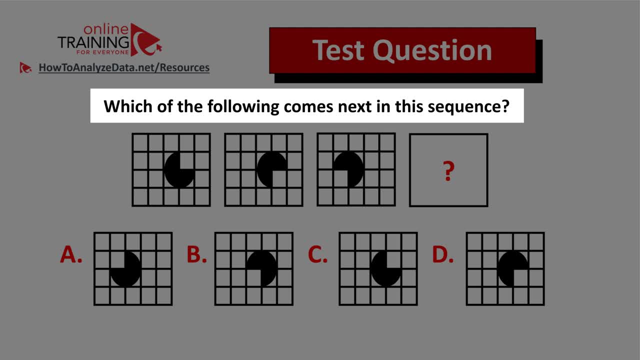 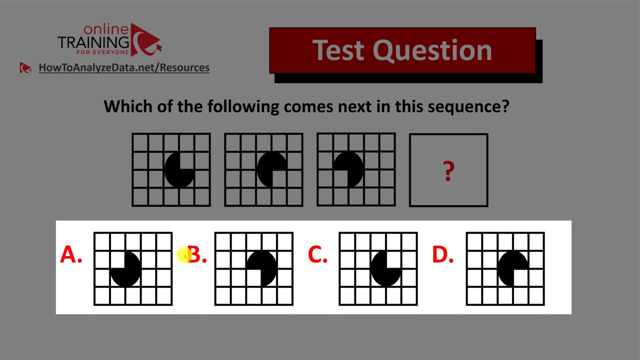 skills. Which of the following comes next in the sequence? And you have a sequence of 4 by 5 rectangles and each rectangle contains a pi inside of the rectangle. The figure 4 is missing and there are four different choices for you to select from: Choice A, B, C and D. Now might be. 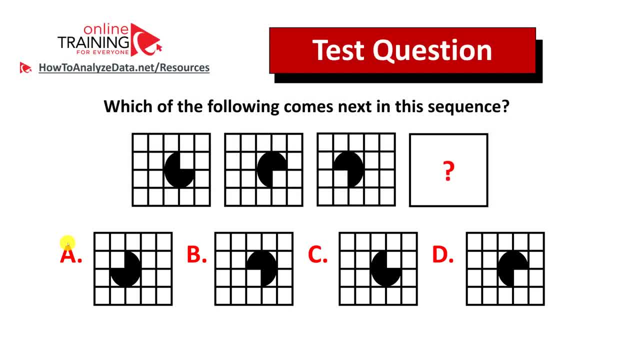 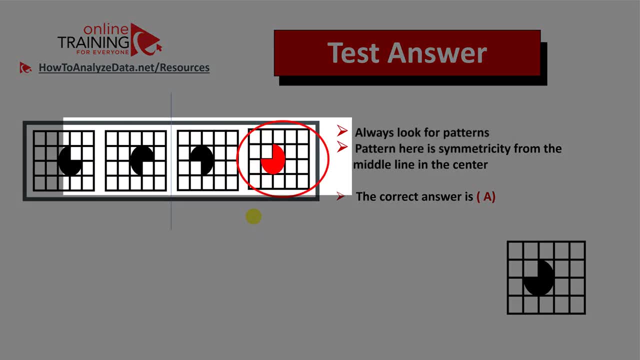 a good time to pause this video to see if you can come up with the solution on your own. Did you figure out the answer? Let's continue to see how we can get to the answer. As usual, my advice is always the same: Always look for patterns. And here the pattern is. 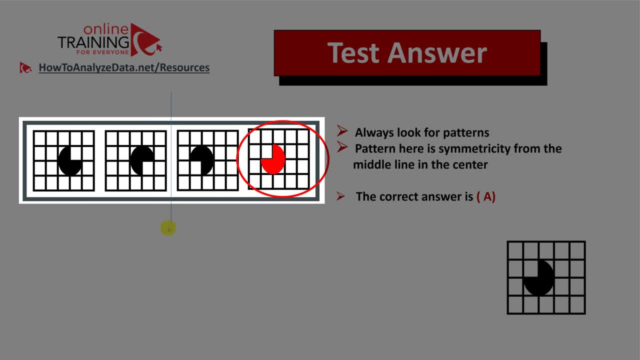 symmetricity. You see, if we draw a line in the middle, you can see that the shapes, the pi pieces, are symmetrical. You see the pi in the first square which mirrors the pi in the last square, because the pi's in the second and third squares are also mirrored. Hopefully you've nailed this. 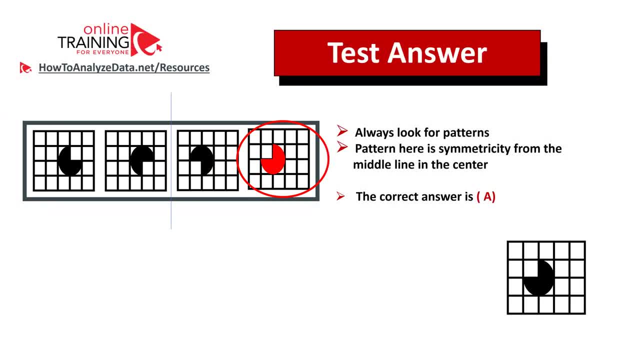 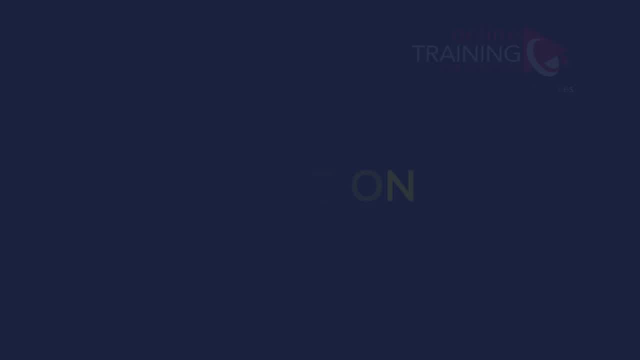 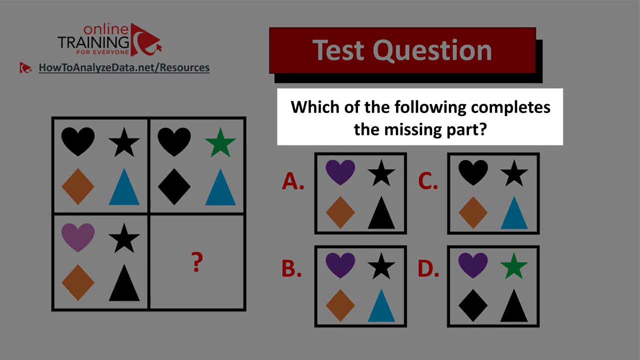 question and now know how to answer similar problems on the test. Let me share with you a tricky question which tests your reasoning, analytical as well as visualization skills. Which of the following completes the missing part? And you're presented with a 2 by 2 box. One of the squares in the big box is missing and you have four different. 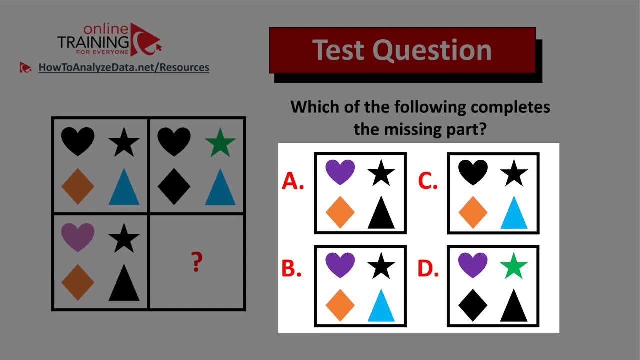 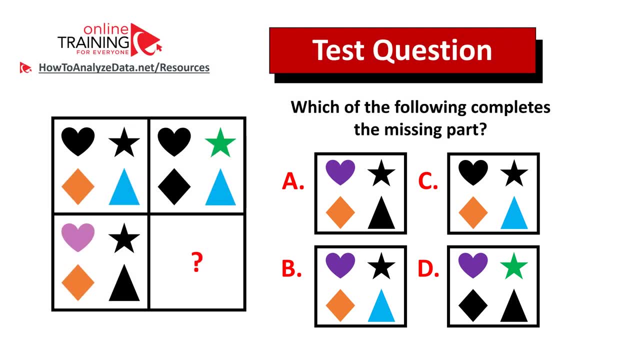 choices to choose from A, B, C and D. Take a closer look and see if you recognize the pattern. Do you think you know the answer? Now might be a good time to pause this video to see if you can come up with the solution on your own. Give yourself 10 or 20 seconds to see if you can come up with. 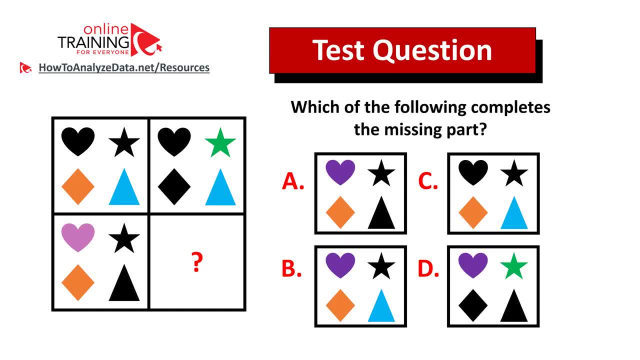 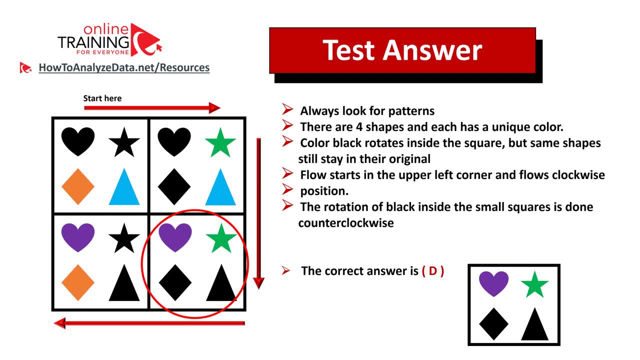 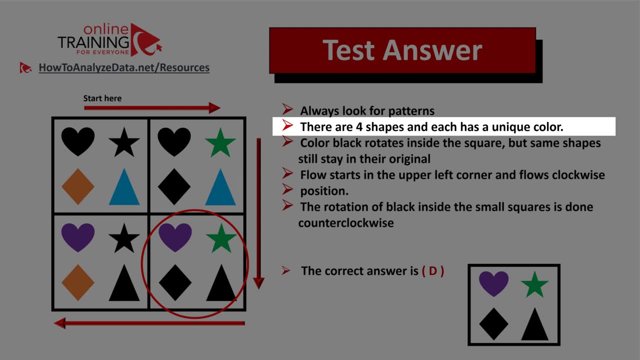 the answer. Did you come up with the answer? Let's continue to see how we can solve this challenge together. Tricky question, isn't it? But, as usually, all tricky questions always have the answers. So take a look here. There are four shapes inside the square, and each shape has a unique color. 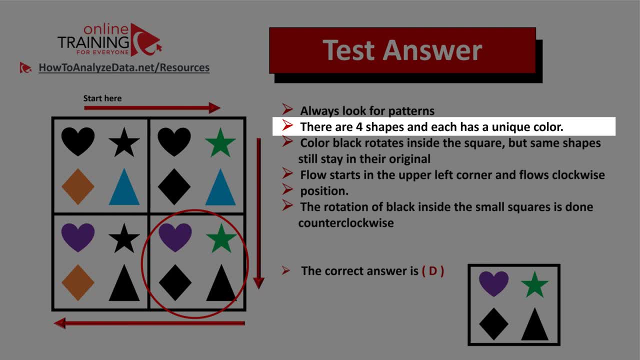 Shapes stay in place. The only thing that changes is the black color for the shape, And what you can see is that the pattern of the black colors inside the squares, and it rotates counterclockwise. So, as usual, always look for patterns. You see that the flow among the shapes starts in the upper left corner. 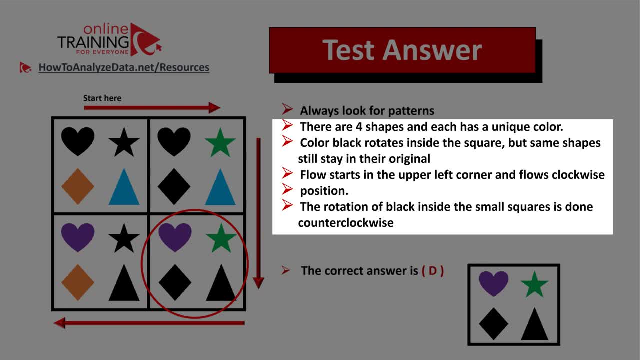 and flow goes clockwise, But the rotation of the black color inside the squares goes counterclockwise. So that's the tricky part of the question, But there's always the right answer And, as you can see, the right answer here is choice D. Let's recap: Always look for patterns. 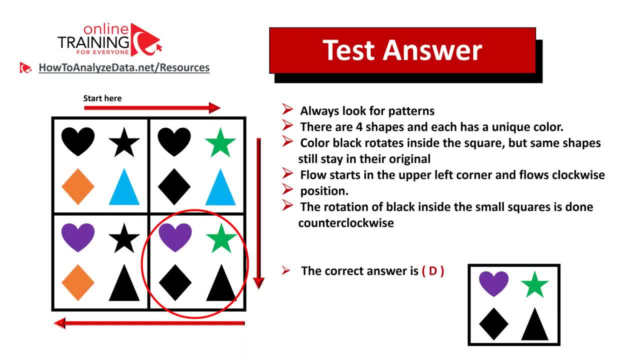 In this case there are four shapes and each shape has a unique color. Color black rotates inside the square, but same shapes stay in their original position And the rotation inside the squares is done counterclockwise. So hopefully you've nailed this question and now know how. 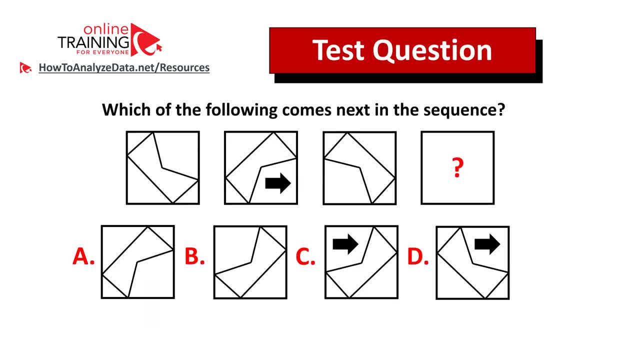 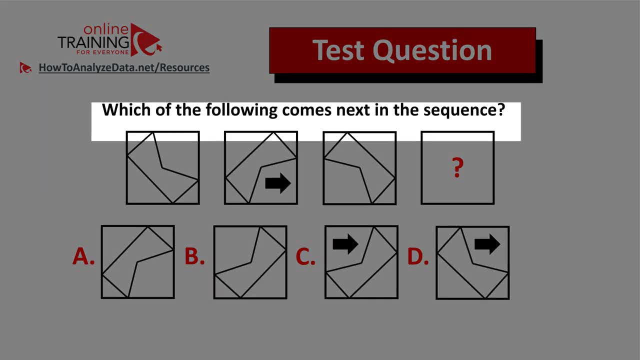 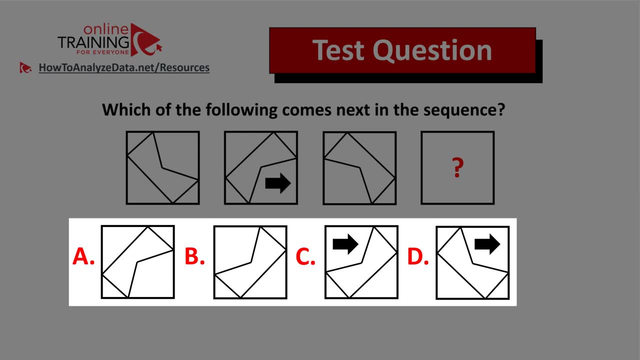 to answer similar problems on the test, And here's the question you can try to solve on your own: Which of the following comes next in the sequence? You are presented with four different squares and each square has another figure inside, And there are four possible choices: A, B, C and D. 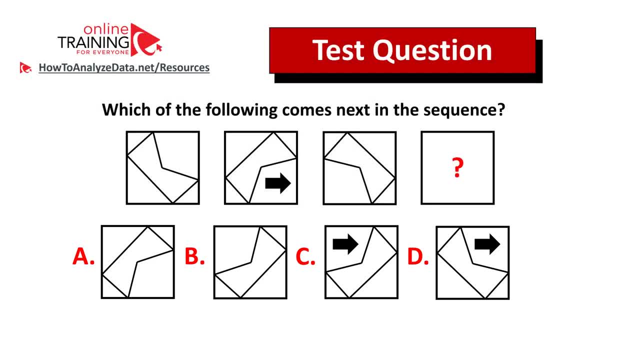 Now might be a good time to pause this video and give yourself 10 to 15 seconds to see if you can come up with the solution. One tip for you: Always look for patterns. If you figured out the answer, feel free to pause the answer in the comment section of this video. 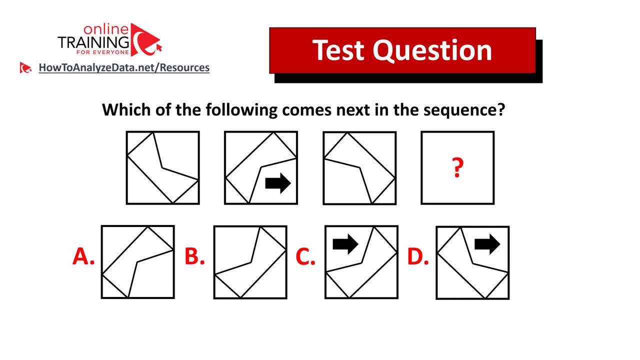 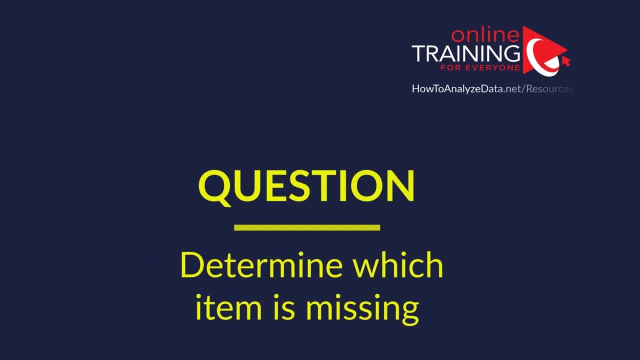 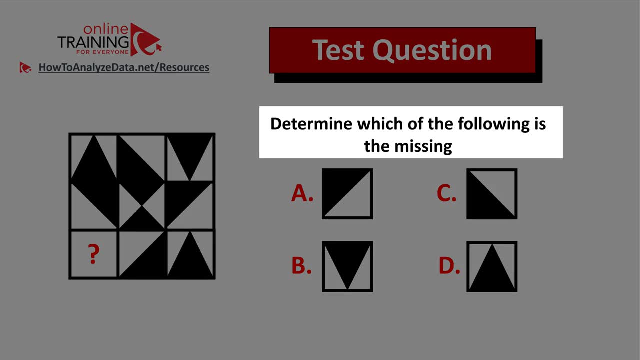 Also, please make sure to post your rationale so I can give you my feedback. Thanks for participating and good luck on this challenge. Let me share with you an interesting question which tests your reasoning skills. Determine which of the following is missing, and you're presented with the large square which could. 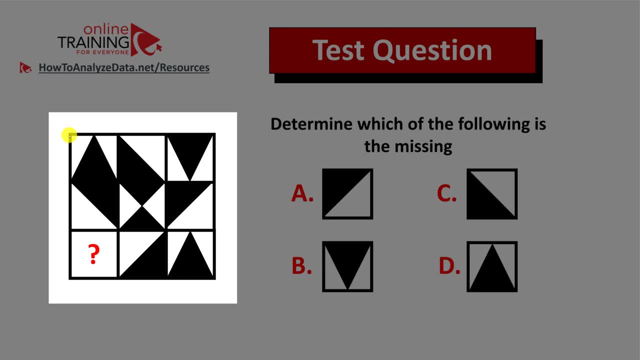 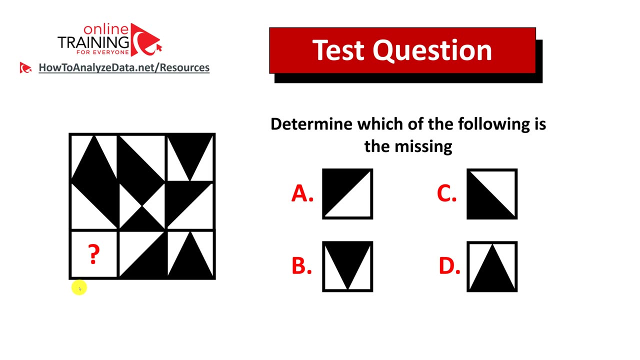 be logically broken into three by three small squares and four different choices: Choice A, B, C and D. You have a missing square in the bottom left corner. Do you think you can figure out the answer? Now might be a good time to pause this video and give yourself 10 to 20 seconds to see if you can. 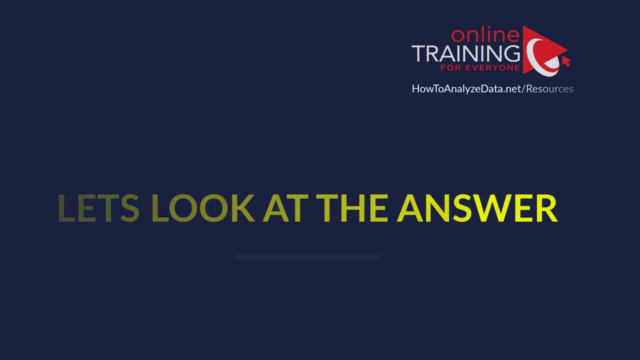 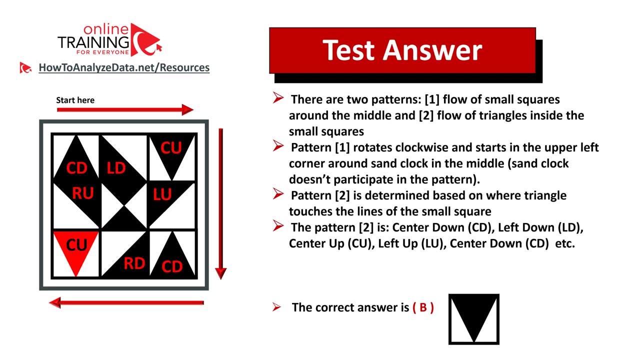 figure out the solution. Do you have the answer? Let's continue to see how we can solve this puzzle and get to the correct solution together. We presented with the very interesting challenge here, but challenge could be broken down into two patterns. The first is an easy one: You must be familiar with the number of squares in the bottom left corner. 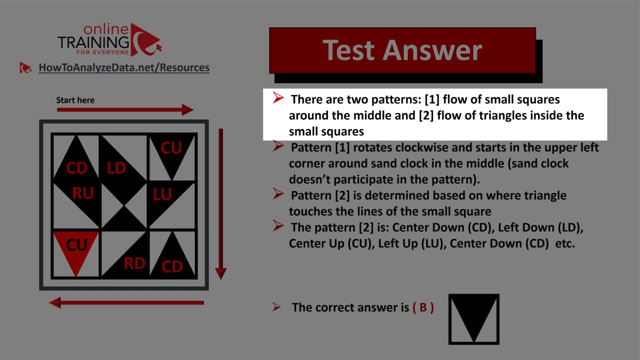 The first pattern is the flow of small squares around the middle and the second pattern is the flow of triangles inside the small squares. Pattern 1 rotates clockwise and starts in the upper left corner. You see that the pattern rotates around the cent clock. 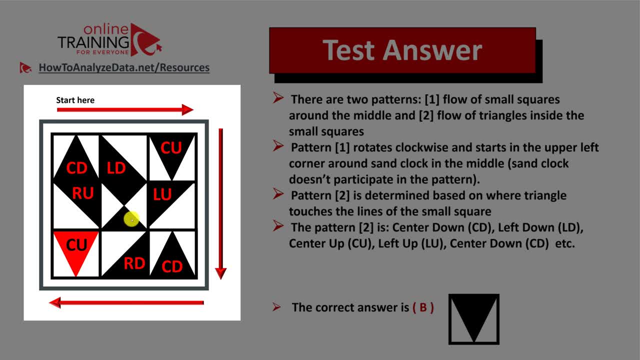 which is in the middle and cent clock does not participate in the pattern. And pattern 2 is determined based on where triangle touches the lines of the small square. For example, the triangle in the upper left corner touches the lines of the small square in the center. 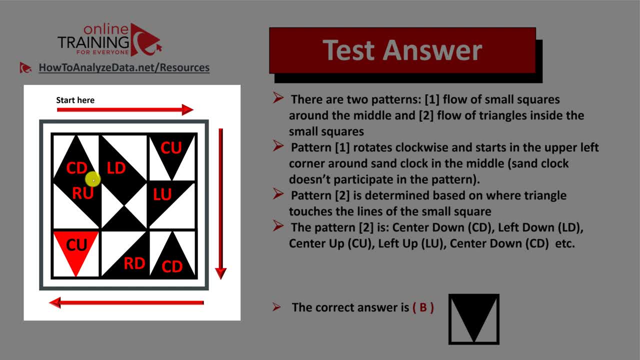 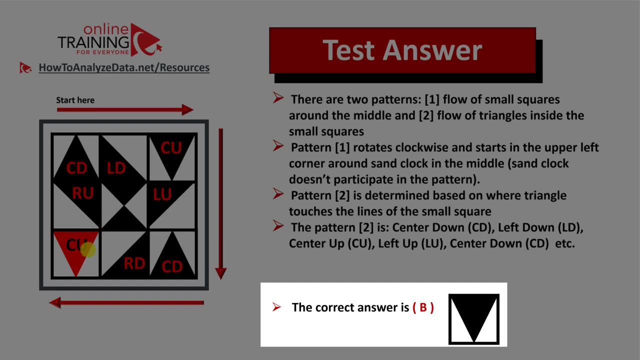 you see on the top as well as down. at the bottom, Next one touches on the left and down, The following one touches in the up and also in the center, And you can continue this pattern to determine the missing item, which is choice B. 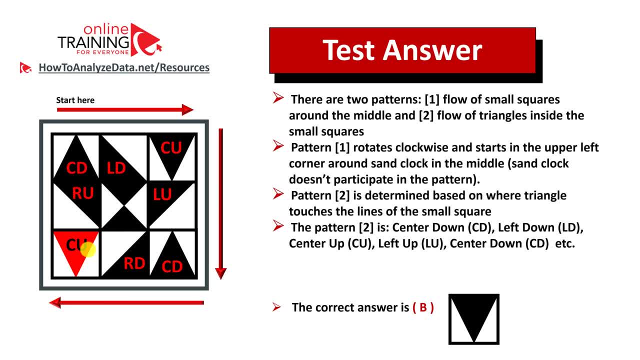 It was a tricky question but I hope by now you know what to look for and how to answer similar problems on the top. But in case you need more questions or practice problems, please make sure to check out my e-book in the description section of this video. 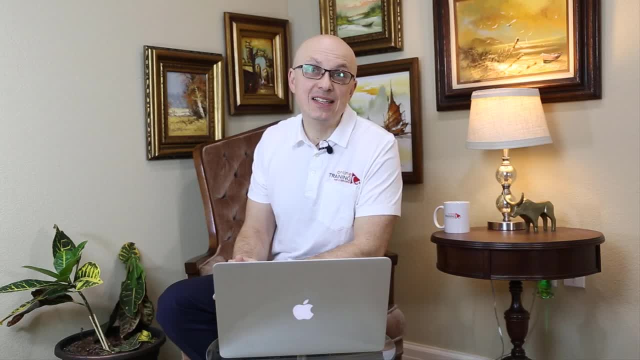 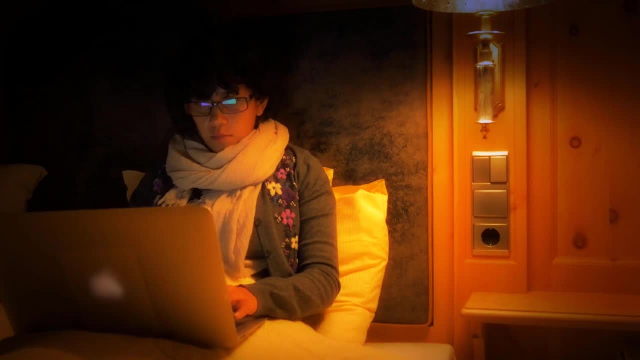 Let's take a look at some considerations when you take an employment assessment test from home. A lot of tests are being conducted from home today. Let me give you some tips: how to succeed on the home-based test and get the best score. Number one: 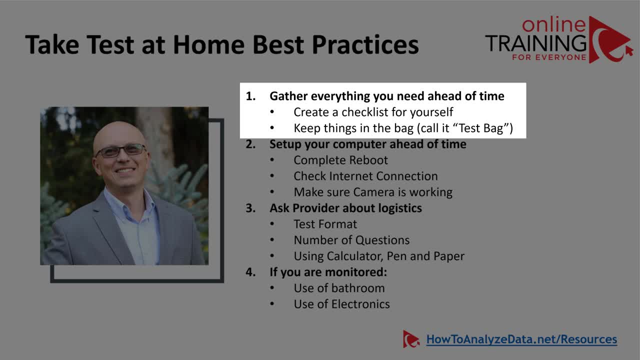 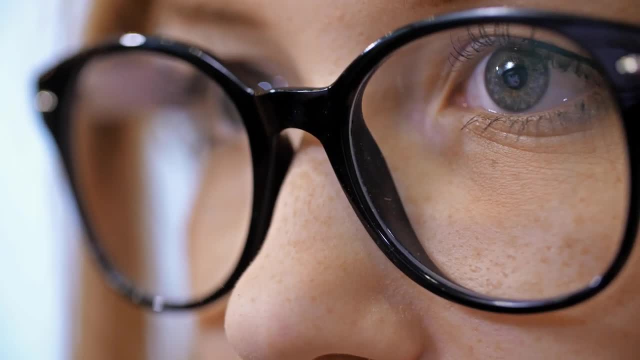 you want to gather everything you need ahead of time and organize yourself. Create a checklist of what you might need if you're taking an employment assessment test from home, And then keep things in your bag- Maybe call it a test bag or test location- from where you can just grab all these things that you need and put them on the table. 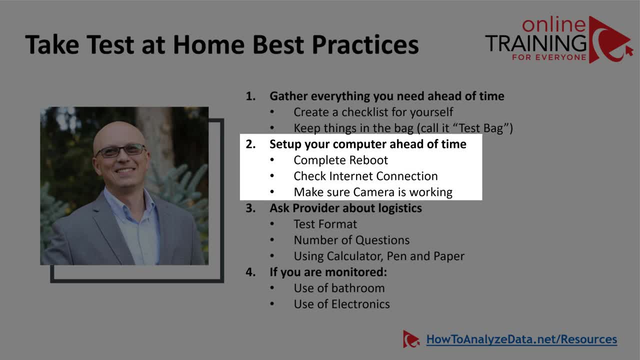 Another important thing is consider setting up your computer ahead of time. Can you complete the reboot of your computer, close all the applications, Make sure you check internet connection, Make sure your camera is working, as most of the time you will be monitored. You can also ask provider about logistics. What is the test format? Is it multiple choice questions? 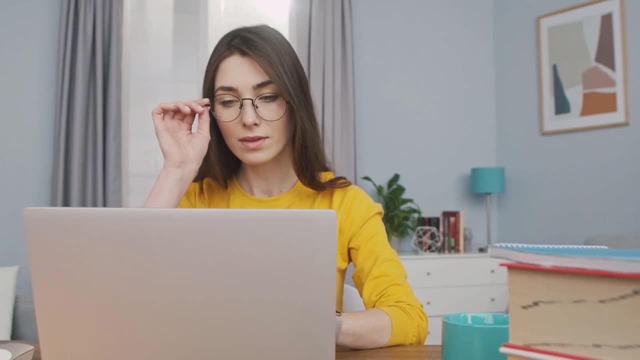 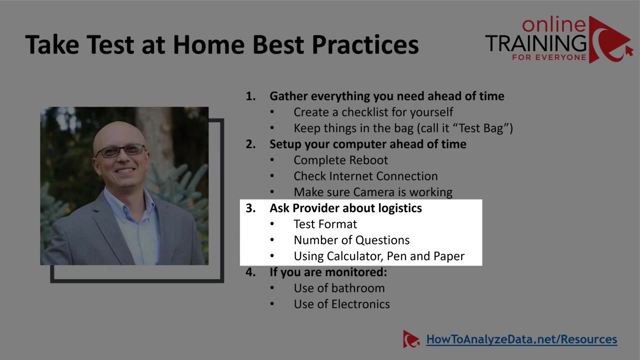 Would you need to do any practice? How many practice exercises? How many questions you will have, How test results are gonna be scored And what is the passing score, if any? You can also ask about using the calculator, using pen or paper. Is it allowed? 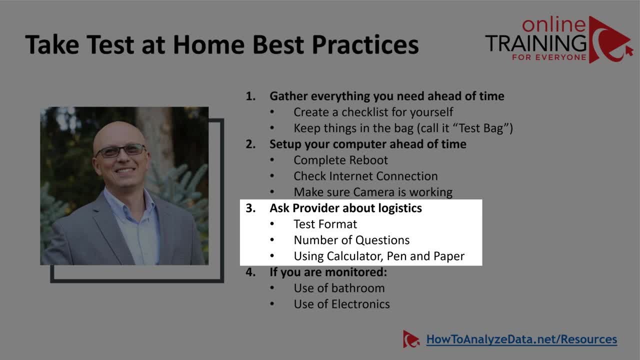 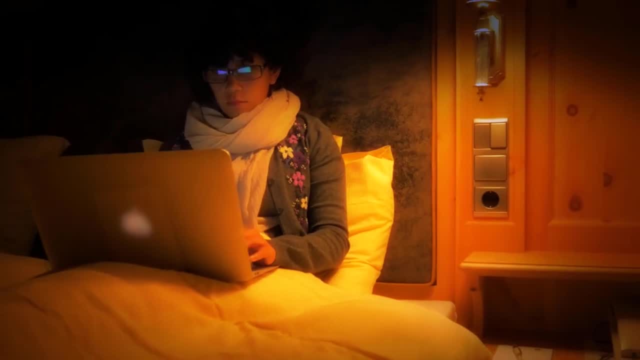 Some test providers may not allow for you to use any one of those. And, last but not least, if you're monitoring, how do you use a bathroom? A lot of times when you're monitored, companies provide you with unlimited test duration, But you need to check. how can you use bathroom to make sure? 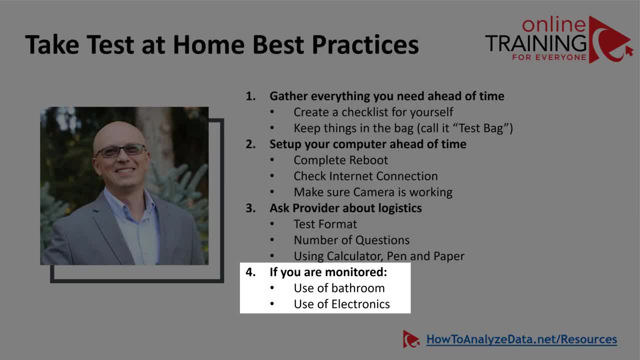 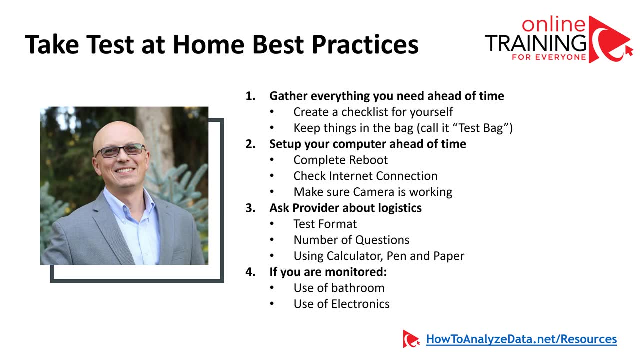 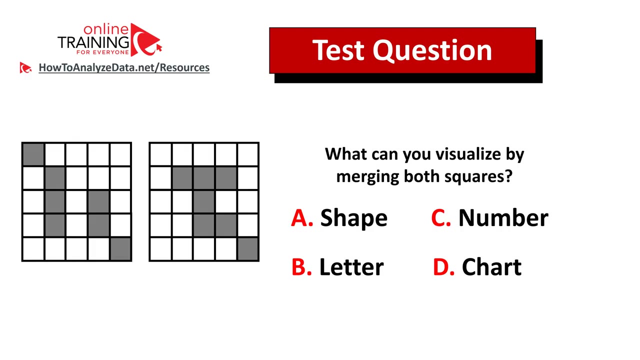 your test results are not invalidated. Also, if somebody calls you or texts you, how would you respond to those? Checking those things ahead of time helps you succeed on the test. Here is the question from the real test, But somehow I have a feeling that you. 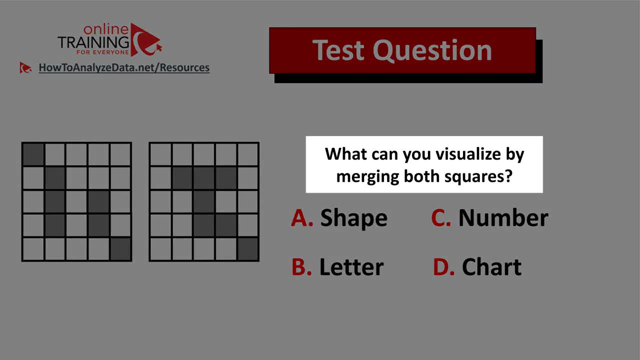 might come up with the answer. What can you visualize by merging both squares? You're presented with five by five squares on the left And you have four different choices to answer this question. And you have four different choices to answer this question And you have four different choices to answer this question. 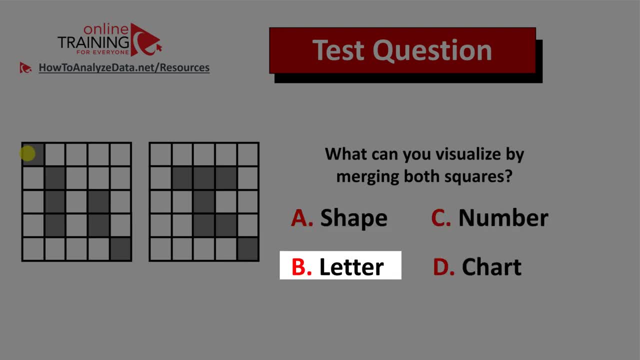 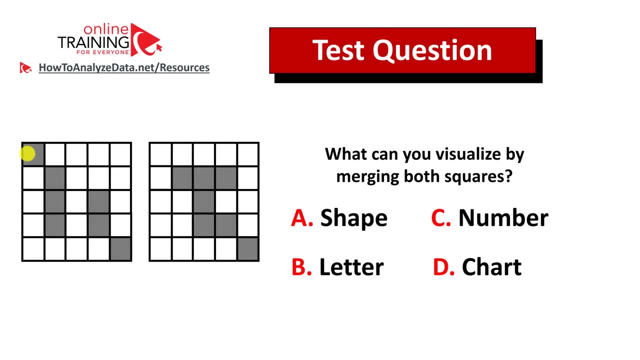 Choice A shape, Choice B letter. Choice C number And choice D chart. Do you see the answer? Give yourself 10 to 15 seconds. maybe pause this video to see if you can come up with the answer on your own. 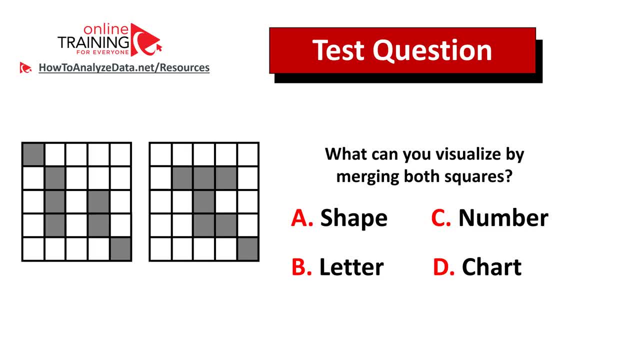 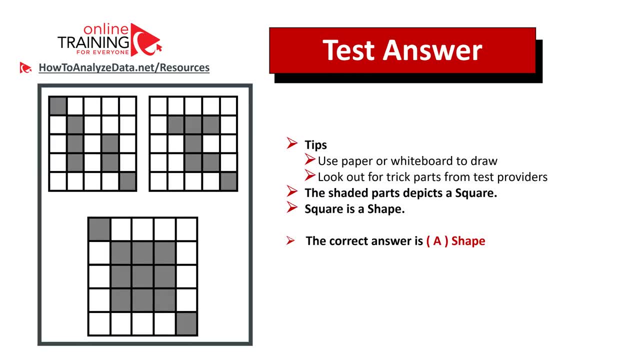 Did you figure out the solution? Let's see how we can solve this challenge and get to the correct solution together. Before jumping to the solution, let me give you a couple tips. If you have access, please, please use the paper or whiteboard. 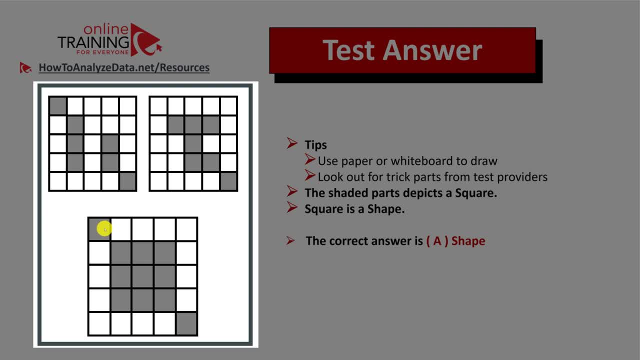 If you have access, please, please use the paper or whiteboard to draw this shape and see what can you come up in the final figure. This is necessary because our brain- at least mine- is not very well designed to visualize particular figures. 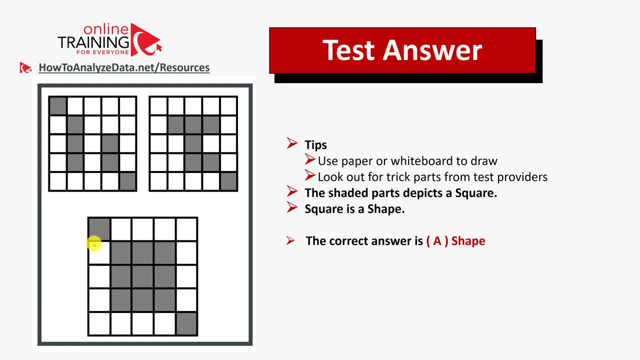 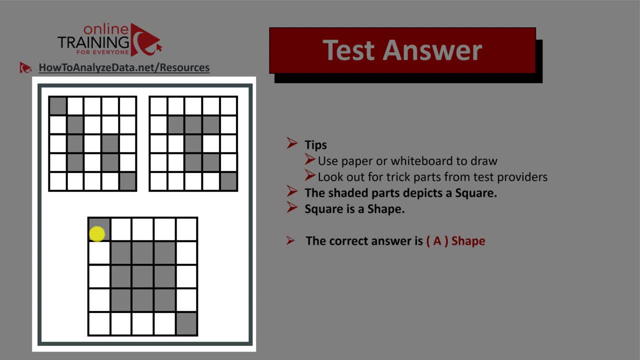 So maybe you are different or maybe you know better solutions. In this case, if you have the ability to visualize, you're very lucky, because most of the people don't have this ability. They should be using paper or whiteboard to get to the certain answer. 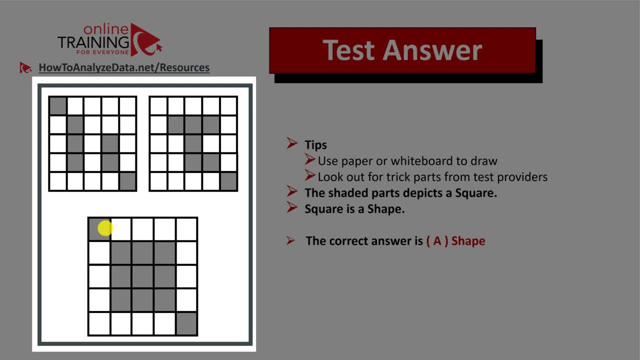 Another tip here is look out for trick parts that might be included into the final shape upon merging, and they are created by test providers to confuse you. As you can see, upon merging both squares in the top, you see the final square at the bottom. 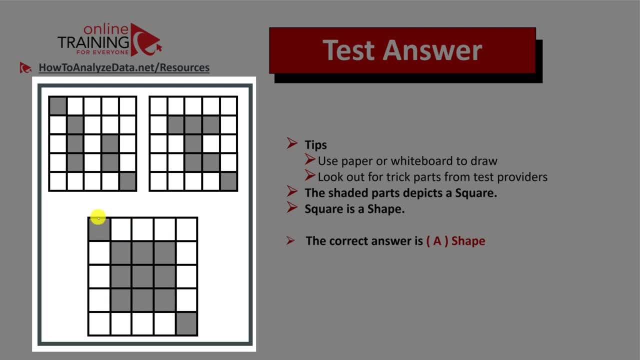 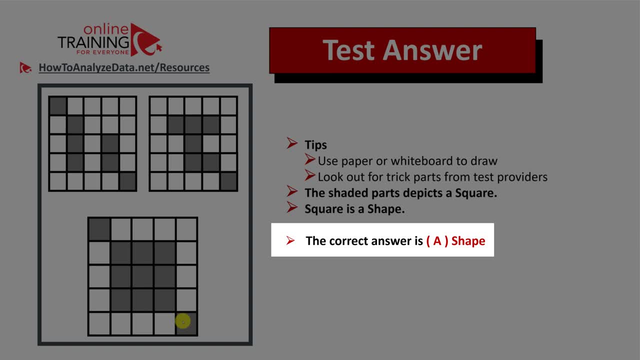 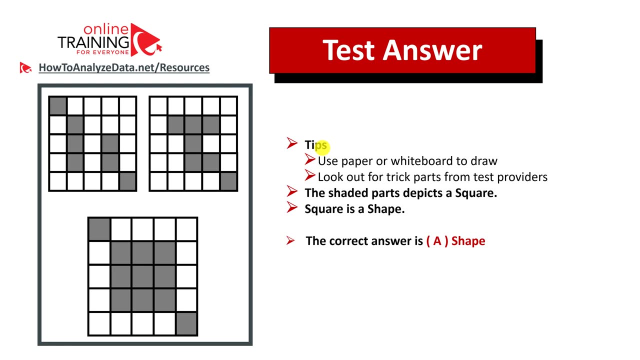 And you see that there is a square in the middle, as well as two shaded small squares in the upper left corner and in the bottom right corner. So the correct answer here is choice A shape, because square is the shape. But make sure to use those tips I shared with you earlier to increase your chances of answering these types of questions correctly. 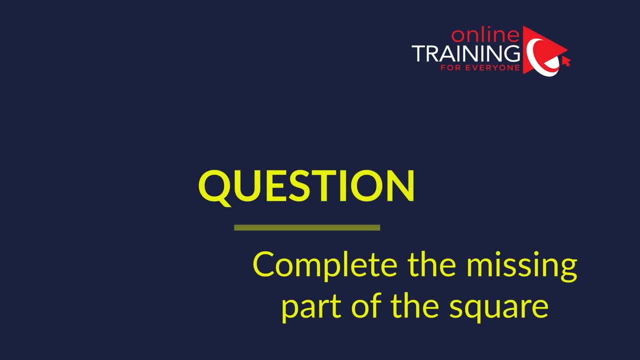 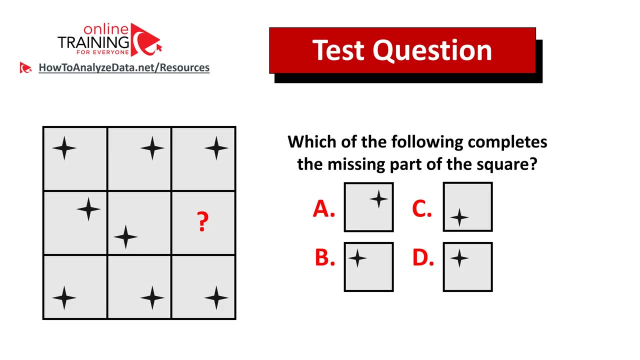 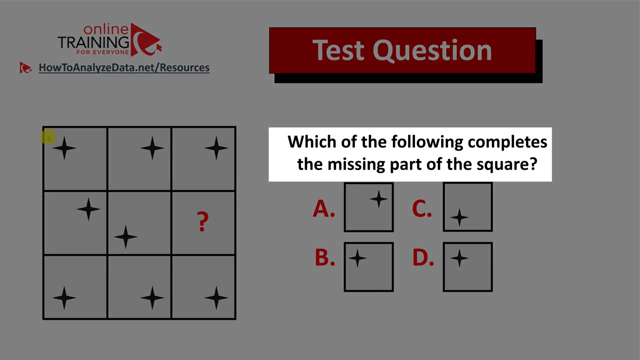 Let me share with you a tricky question from the test. Somehow, though, I have confidence that you might figure out the answer. Here's the question: Which of the following completes the missing part of the square? And you have a 3x3 square which consists of the smaller squares. 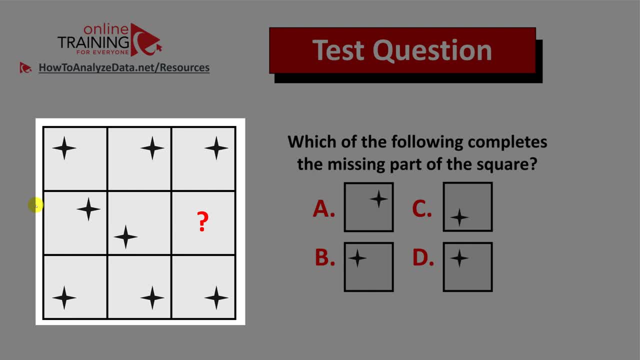 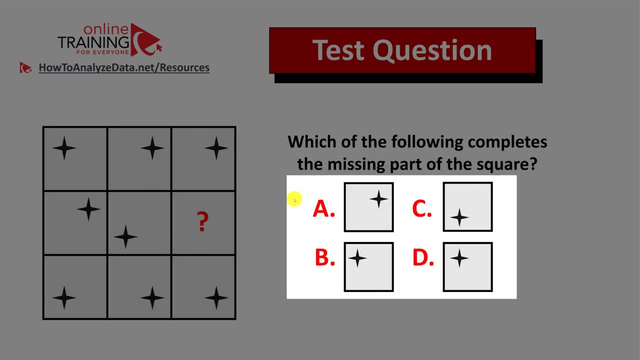 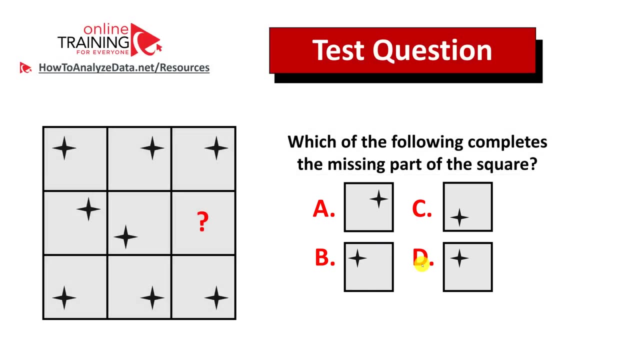 Each small square has a star and all stars are in different corners. One small square is missing and you have four different choices To figure out the final answer: Choices A, B, C and D. Each choice has a star in a different corner. 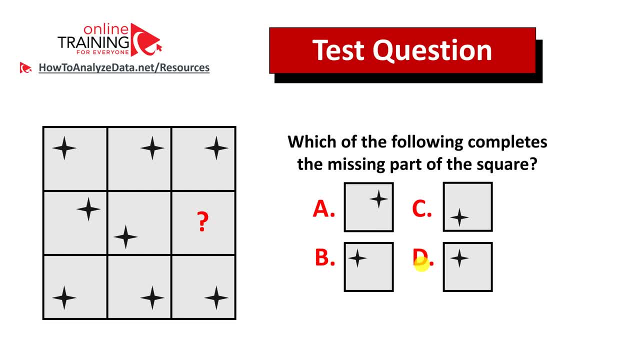 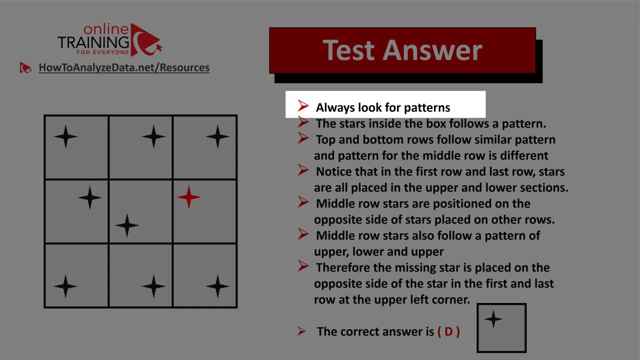 Do you think you know the answer? Give yourself 10 to 20 seconds to see if you can come up with the answer on your own. Did you figure out the answer? Let's go ahead and jump straight to the solution. As usual, the best advice I can give you is always look for patterns. 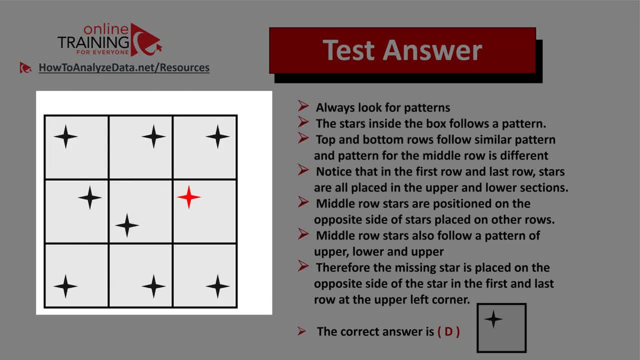 So there are multiple patterns going on. Let's look at each one of them. The first pattern is that the top and the bottom rows follow the similar patterns. You see the location of the stars for the top row. They are on the top. 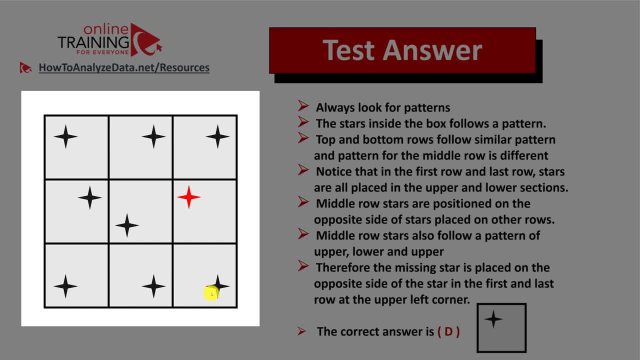 And for the bottom row the stars are at the bottom part of the bottom row. If you follow the middle row, you will see that the stars in the middle row follow a completely different pattern. The first middle row star is at the top, then bottom. 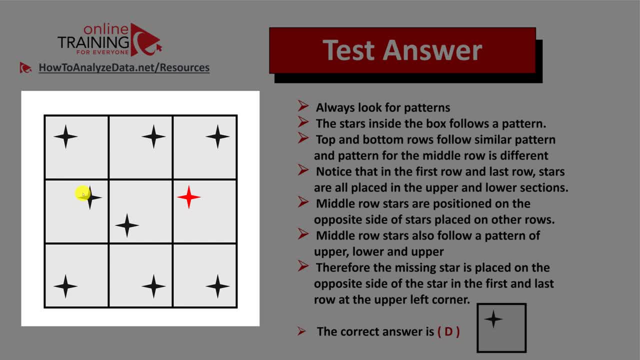 Then the next one logically would be at the top again. You also see that the middle row stars are placed on the opposite sides of the top and bottom row stars. You see in the first column the middle row stars in the upper right corner. 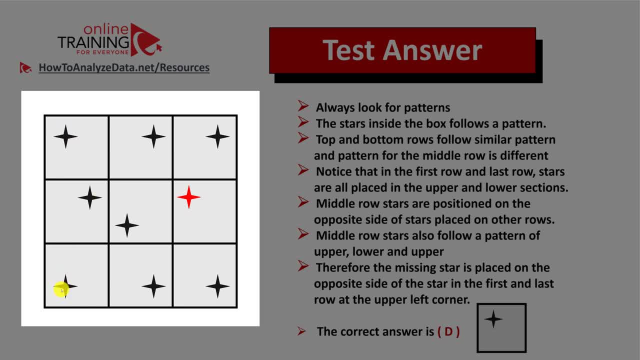 versus the top and the bottom rows, which are placed on the left side. Same thing happens in the middle column And then, assuming that we figured out the pattern, you will see that the same pattern will be applicable in the right column as well. This is why the missing star is placed on the opposite side of the stars. 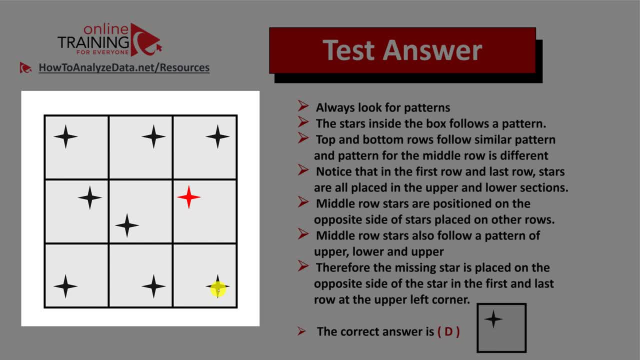 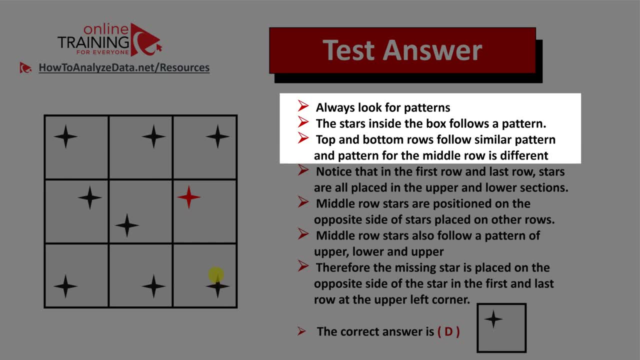 of the stars in the top and bottom rows. Let's recap: Always look for patterns. The stars inside the box follow the pattern. Top and bottom row follow similar patterns and pattern in the middle row is very different. Notice that the first row and the last row stars are placed in the upper and left sections. 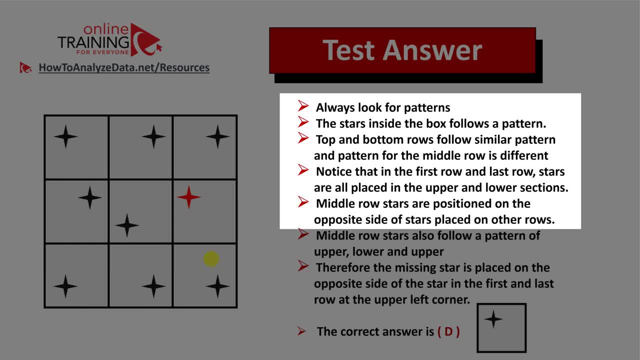 Middle row stars, though, are positioned on the opposite side of the stars placed in other rows. Middle row stars also follow a pattern in the upper, lower and then upper. Therefore, the missing star is placed on the opposite side of the star in the first and last row, at the upper left corner. 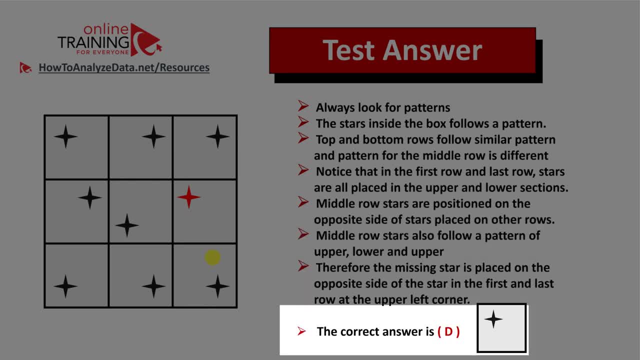 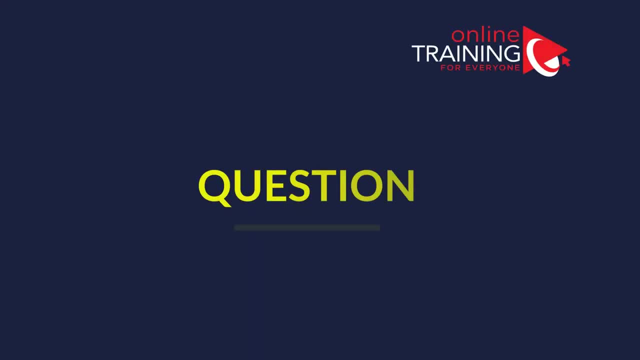 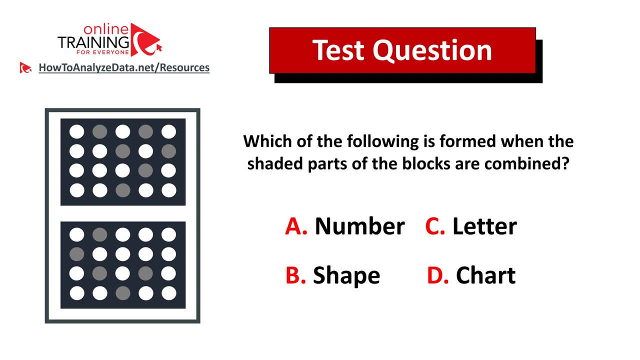 So the correct choice here is choice D. Hopefully you've nailed this question and in case you didn't, you know how to answer similar problems on the test. Here's the tricky question from the real test, But somehow I have a feeling that you might come up with the answer on your own. 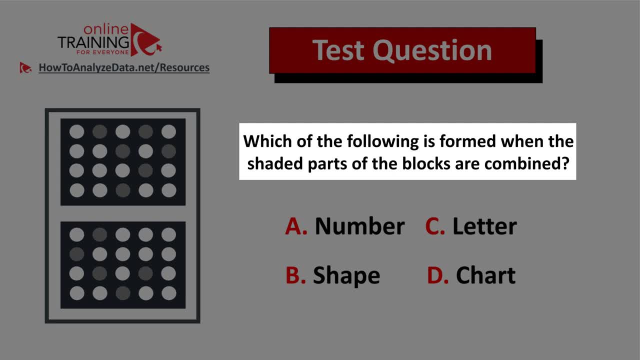 Which of the following is formed when the shaded parts of the blocks are combined And you have four different choices: Choice A- number, Choice B- shape, Choice C- letter And choice D- chart. On the left, you're presented with two blocks. 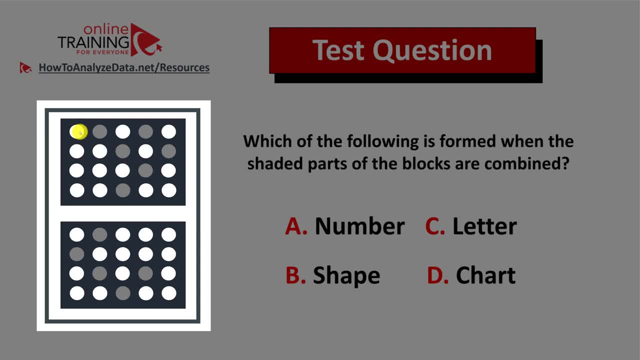 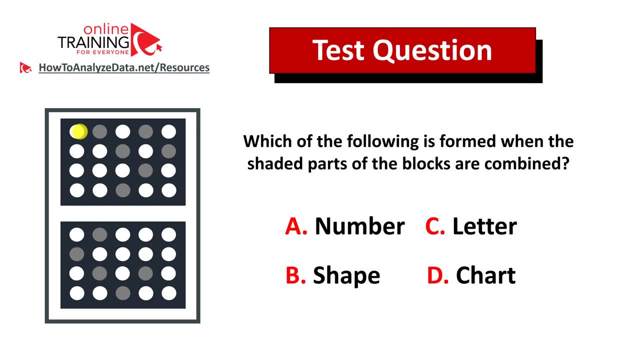 There are two 4x5 blocks and each block has white and shaded circles. See if you can come up with the answer and determine what happens when all these blocks are combined. Give yourself 10 to 20 seconds to see if you can come up with the solution on your own. 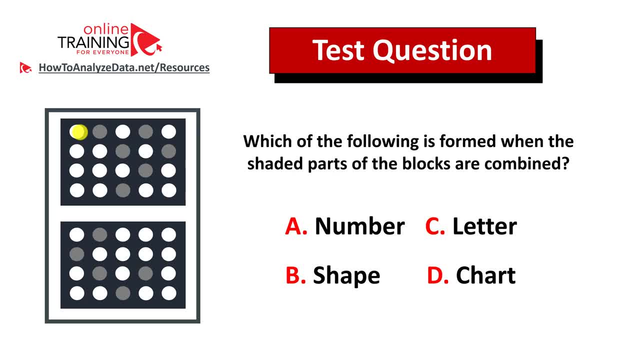 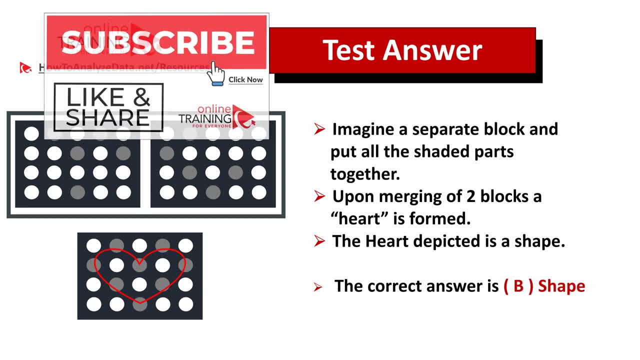 Did you figure out the answer? Let's continue to see if we can solve this challenge together. The best way to solve these types of questions is to imagine a new block and understand what is formed when all the shaded circles are merged together from two original blocks. 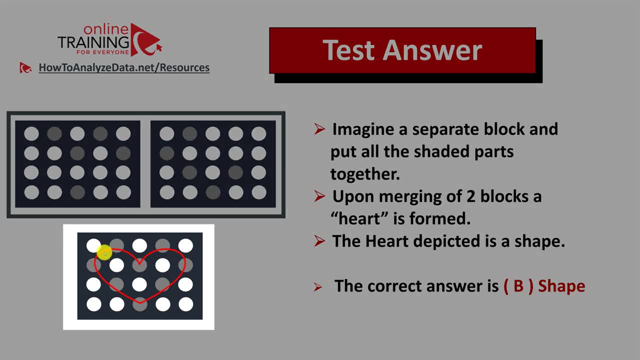 And upon merging you will see that the heart is formed, which is represented here in the third block, And heart is a shape. so the correct answer here is choice B, shape. Hopefully you've nailed this question and now know how to answer similar problems on the test. 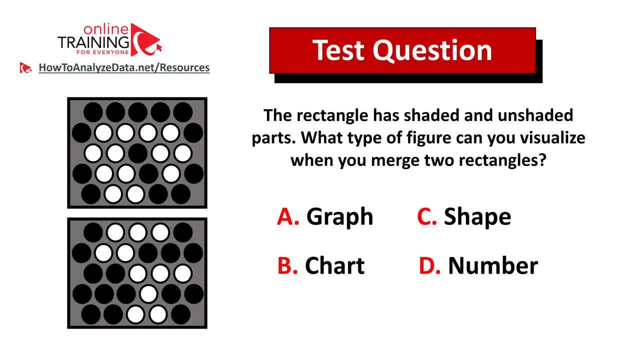 Alright, this question is very interesting and tricky, and you might frequently see these types of questions on the test, But in this case, I'm going to show you the solution and I truly hope that, upon learning, you would know how to solve these questions on the test. 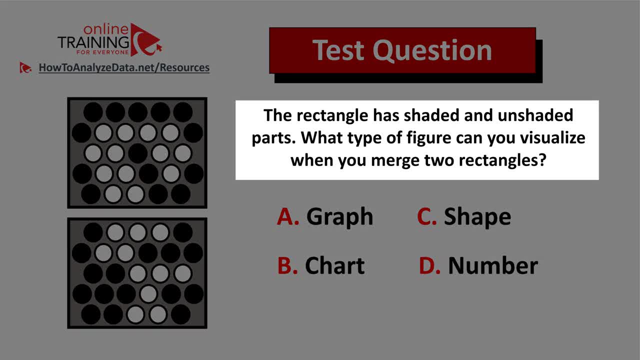 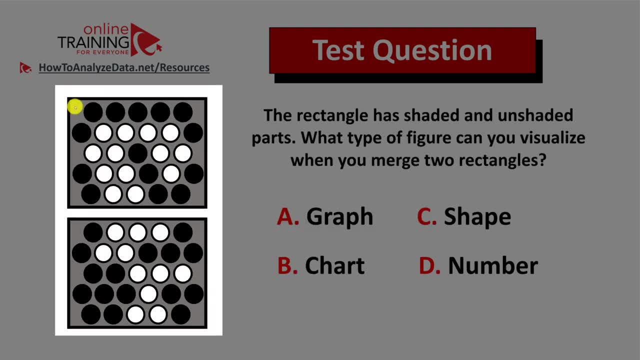 Here's the question. The rectangle has shaded and unshaded parts. What type of figure can you visualize when you merge two rectangles? You have two rectangles on the left. They have shaded and unshaded parts represented by white circles and black circles. 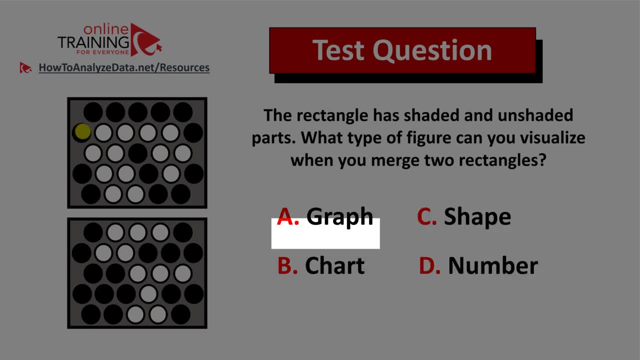 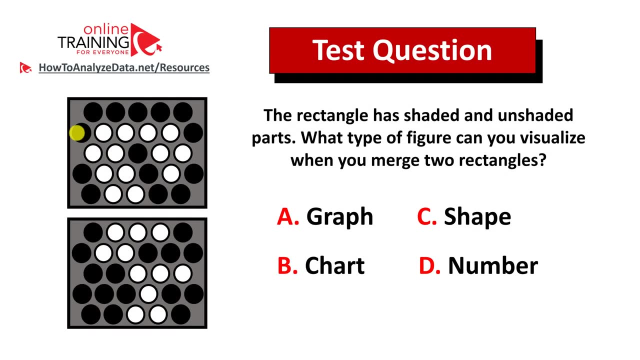 And you have four possible choices: Choice A- graph, Choice B- chart, Choice C- shape And choice D- number. Do you think you know the answer? Let's continue. Please give yourself 10 to 15 seconds to see if you can come up with the solution on your own. 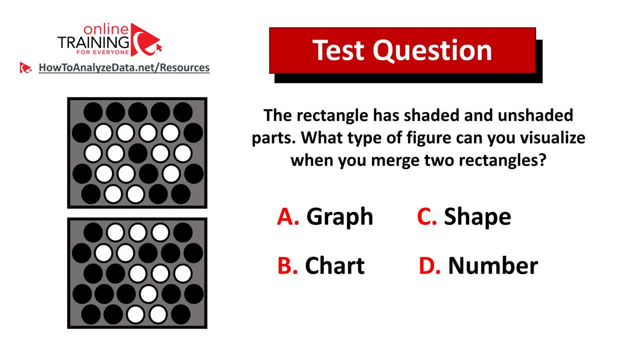 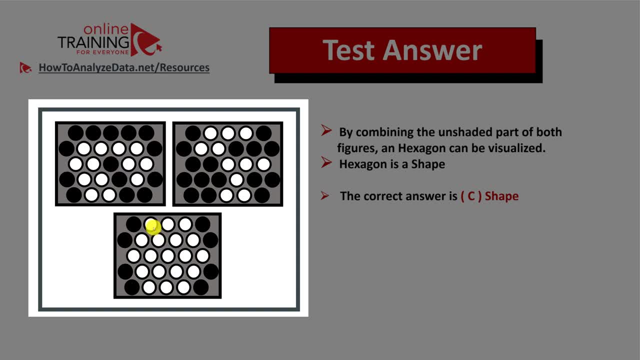 Did you figure out the answer? Let's continue to see how we can solve this question and get to the correct solution together. What you see here is that, upon combining, you can imagine the hexagon, because hexagon is the shape in the bottom rectangle. 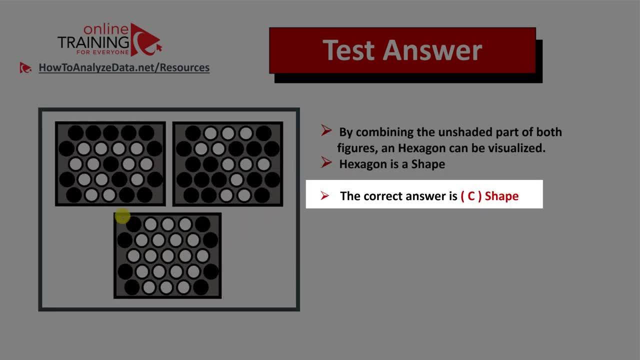 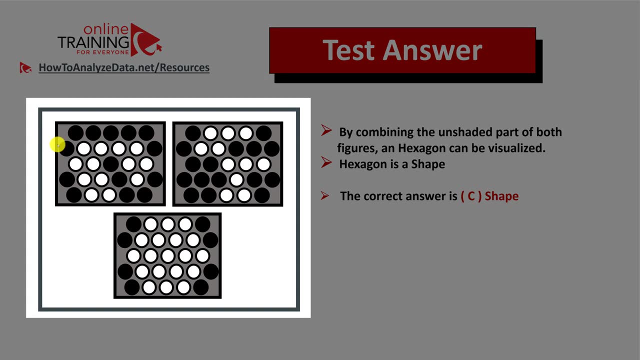 And because hexagon is the shape, the correct answer here is choice C. The trick here is try to visualize it in your head, which is quite hard, But in case you have access to papers or whiteboard, try to take advantage of this. 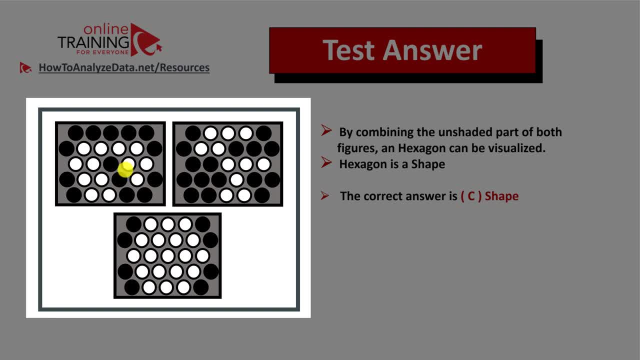 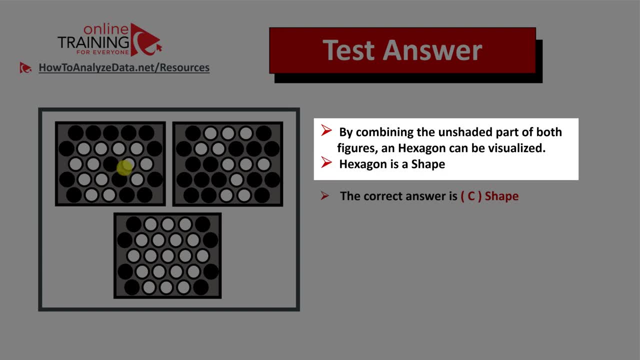 and maybe verify your answer using those tools. Let's recap By combining unshaded parts of both figures, a hexagon can be visualized And hexagon is the shape. So the correct answer here is choice C. Hopefully you've nailed this question. 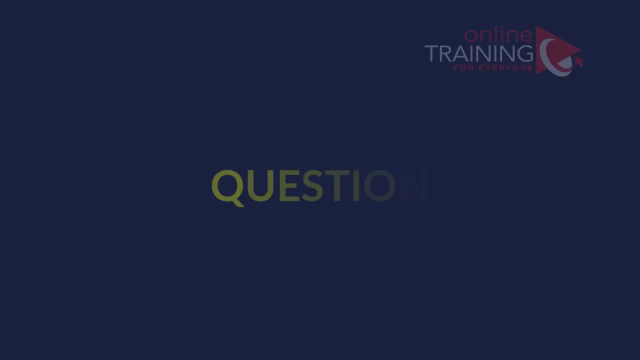 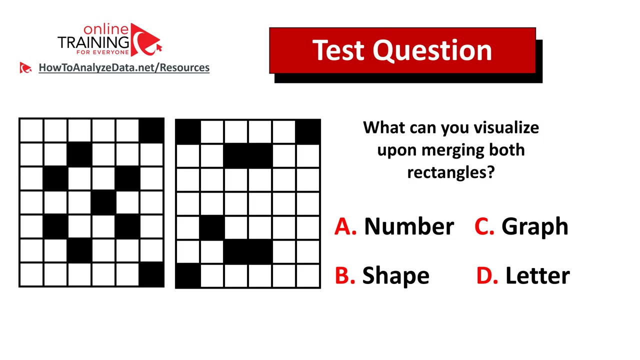 and now know how to answer similar problems on the test. Some of you might find this question tricky, But regardless of whether you can solve it or not on your own, you'll be excited to learn the solution to this real-life assessment test question. 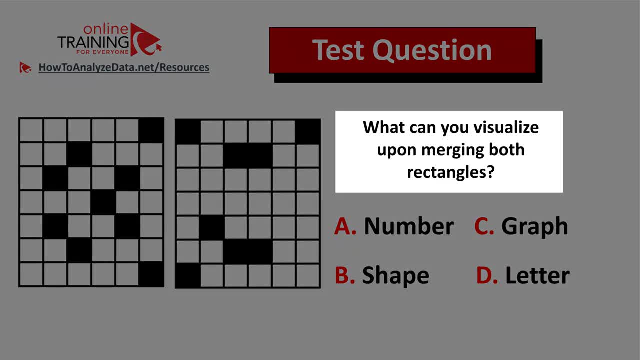 Here's the question: What can you visualize upon merging both rectangles? You're presented with two 7x6 rectangles on the left and you have four possible choices: Choice A- number, Choice B- shape. Choice C- graph, Choice D- letter. 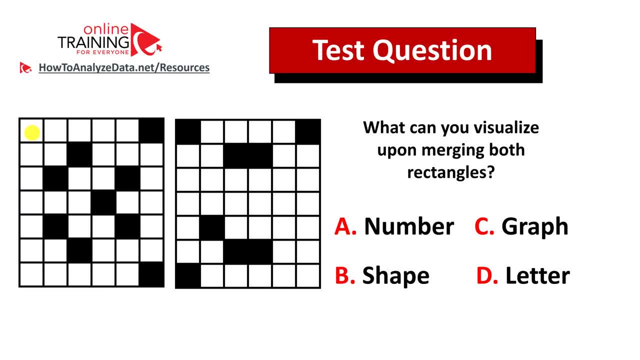 Give yourself 10 to 20 seconds to see if you can come up with the answer On your own. Do you see the answer? Let's continue to see how we can solve this challenge and come up with the correct solution together. As you might be well aware, 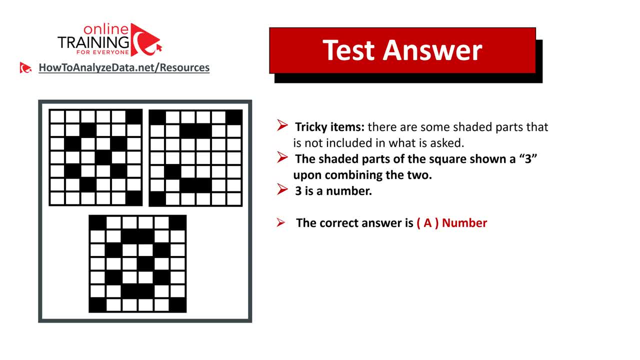 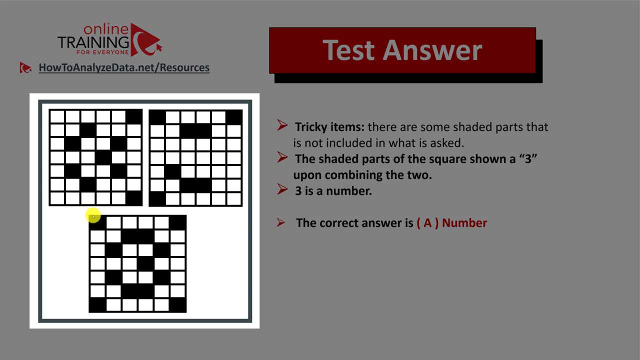 tests are not designed to be solved easily, So you should look out for tricky items as well, And that's what we see here. Specifically, shaded parts in the corners. They're not part of the end figure and they're designed to confuse you. 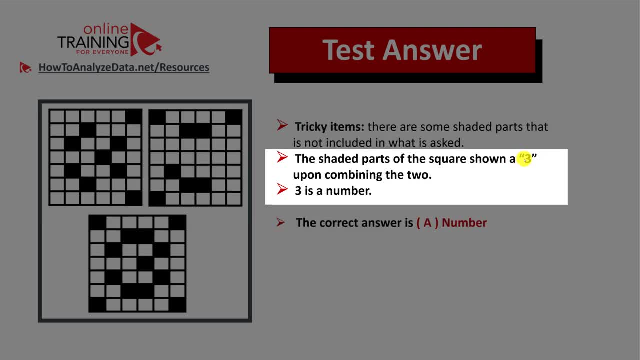 But upon combining both rectangles you can see that you formed a 3 and 3 is the number. So the correct choice here is choice A number, And you can visualize 3 at the bottom rectangle. I'm going to trace it here so you can see it. 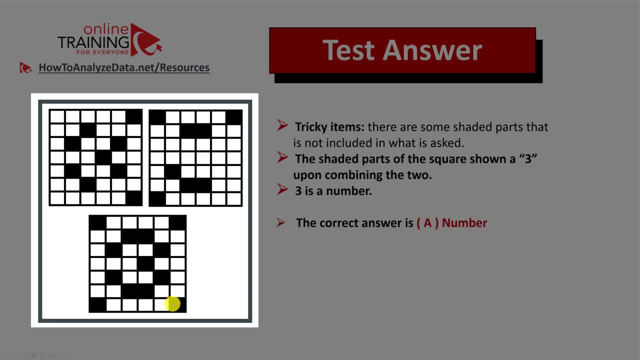 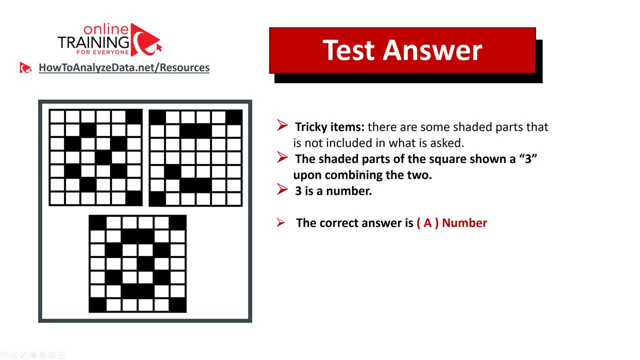 And these are the confusing items right in the corners, So make sure to watch out for those as well. Hopefully you've nailed this question and now know how to answer similar problems on the test. Here's the question from the test you can try to solve on your own. 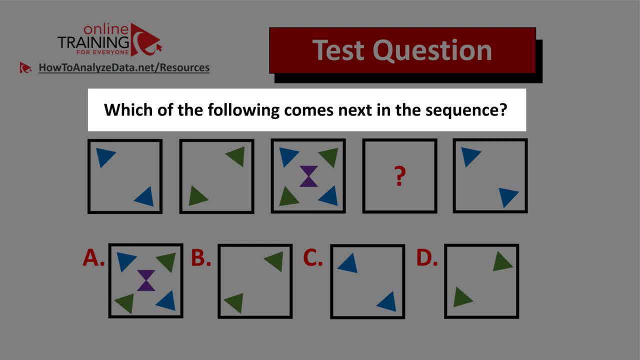 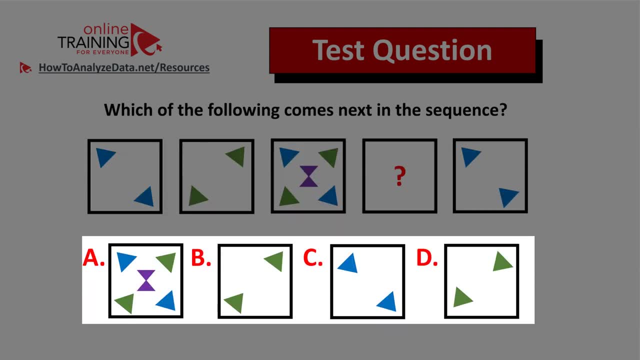 Which of the following comes next? You're presented with the sequence of 5 squares, and square number 4 is missing. You also have 4 different choices to answer this question: Choices A, B, C and D. Do you think you know the answer? 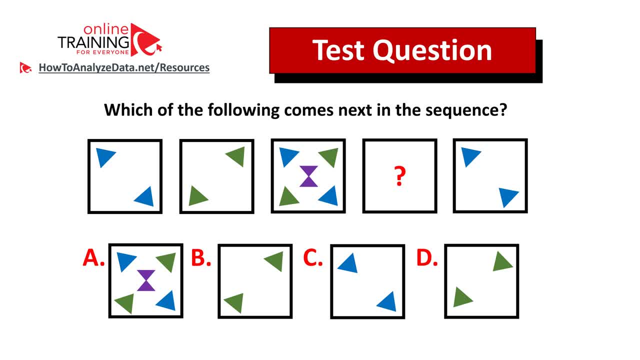 One tip for you here: always look for patterns, And if you figured out the answer, feel free to post it in the comment section of this video, and please provide the answer as well as the rationale. I will also post the detailed answer to this question. 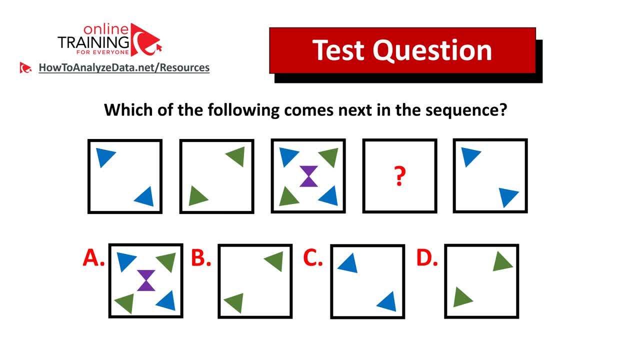 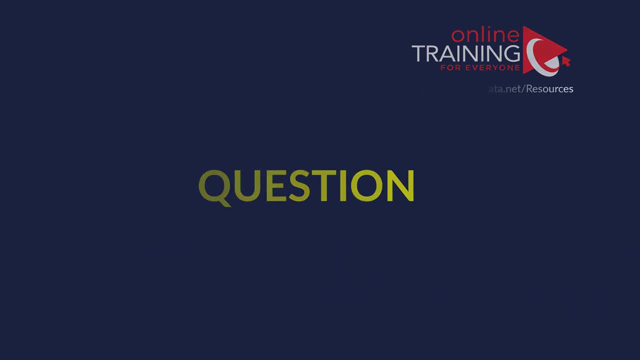 in my future videos. So please make sure to subscribe and review my latest videos on the topic to learn about the answer and how to come up with the answers to similar questions on the test. Thanks for participating and good luck. Here's the tricky question from the real test. 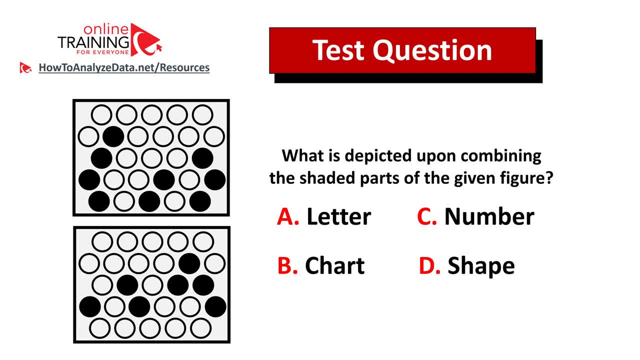 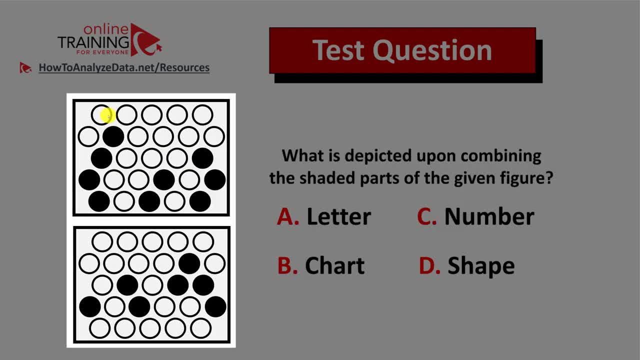 But somehow I have a feeling that you might come up with the answer. What is depicted upon combining the shaded parts of the given figure? And you have two rectangles with circles inside, presented on the left. Each rectangle contains different circles, Some of them are white. 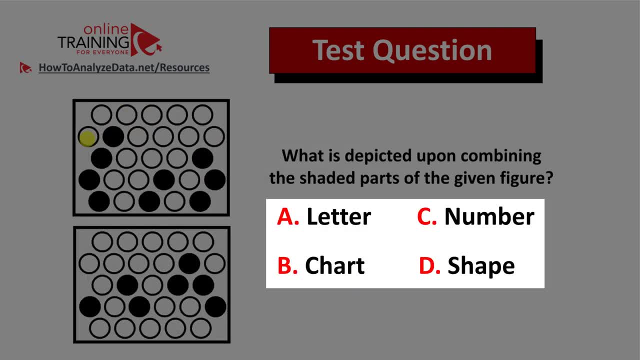 and some of them are filled with black, And you have four possible choices: Choice A- letter, Choice B- chart, Choice C- number And choice D- shape. Can you visualize the answer? Give yourself 5 to 10 seconds. 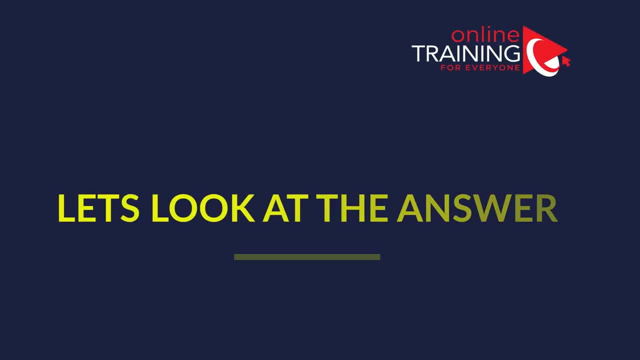 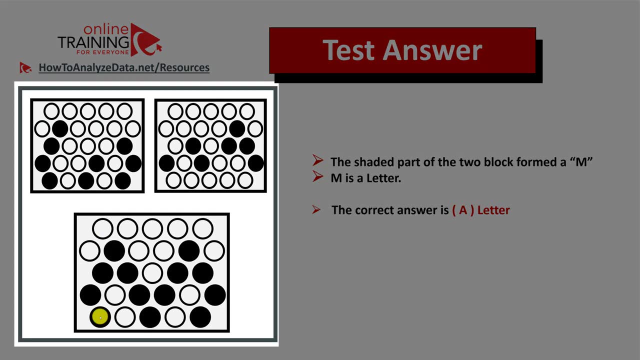 to see if you can come up with the answer. Did you figure out the answer? Let's continue to see how we can get to the correct solution together. As you can see, upon combining two rectangles, M can be formed And M is the letter. 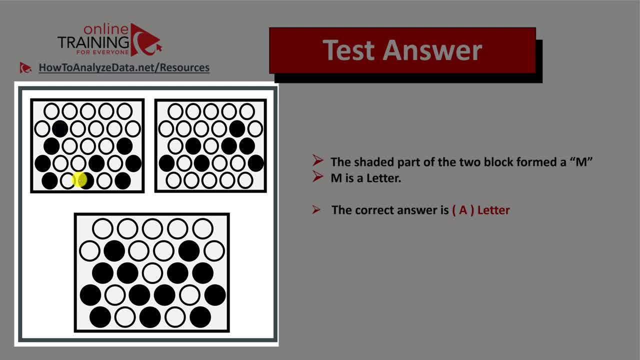 The trick here is that typically during the test, you don't even have access to the paper and you can't depict it on the paper or potentially using any other tools. So you have to visualize this in your memory, And that's the tricky part about this question. 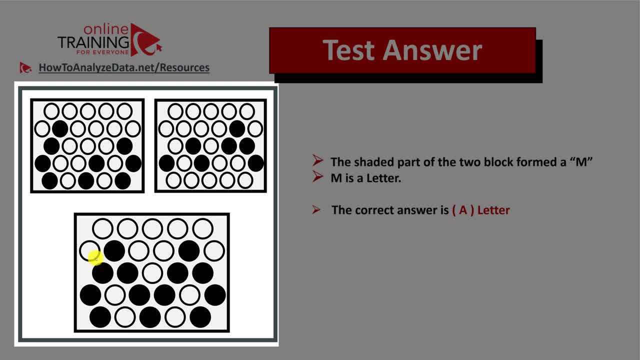 It seems easy once you know the answer. But the trick here is that you need to do it in your head. And what I did- and maybe it will work for you as well- I used the left rectangle as a base And then I moved mentally some of the black dots. 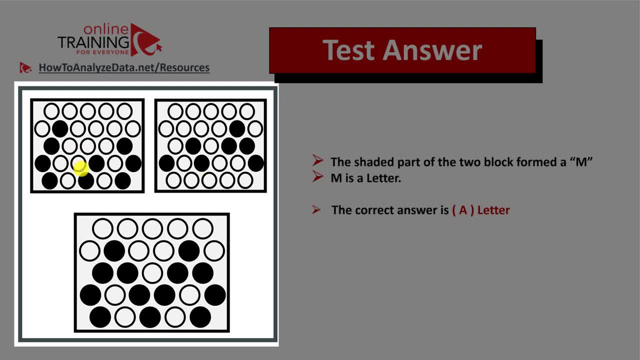 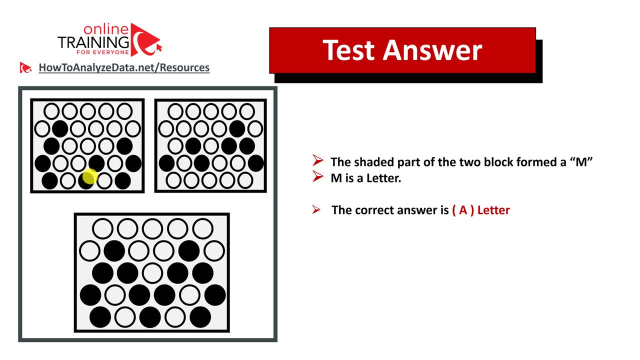 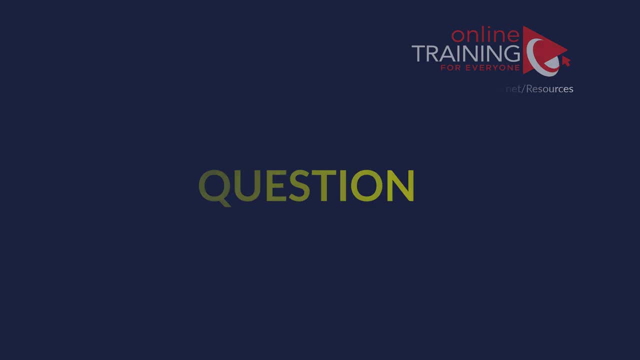 from the right rectangle into the left rectangle to see which shape could be formed, And that's how I came up with the answer M. If you have a better way of solving this, please share in the comment section of this video. Let me share with you a tricky question from the test. 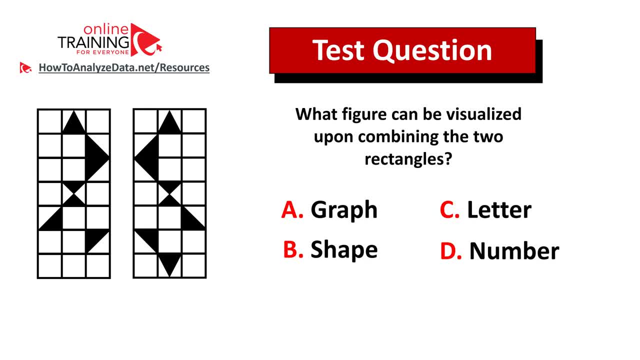 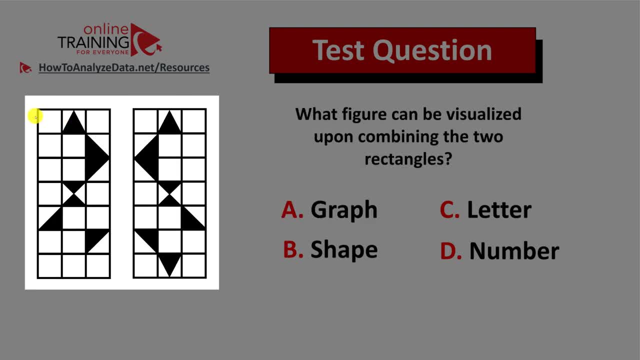 I have confidence, though, that you might figure out the answer. Here's the question: What figure can be visualized upon combining the two rectangles? And you have two rectangles on the left. Both of the rectangles are 7 by 3. And you have four different choices. 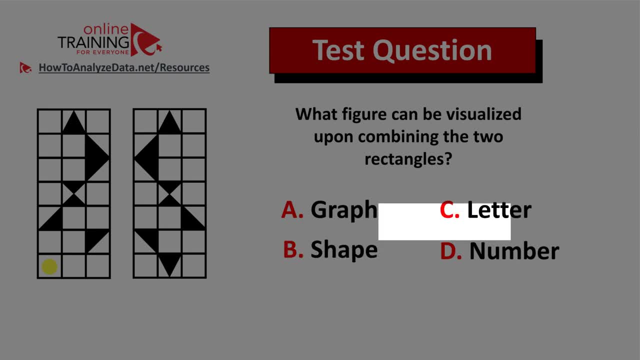 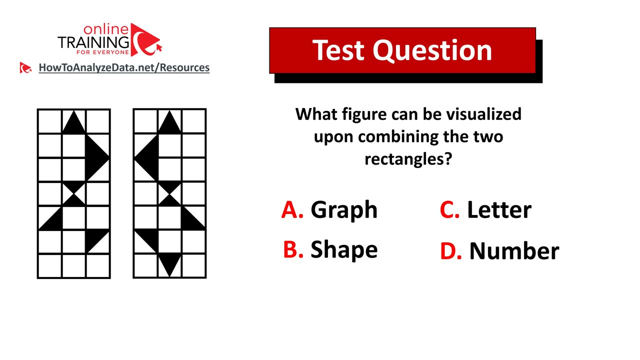 Choice A- graph, Choice B- shape, Choice C- letter And choice D- number. Do you see the answer? See if you can pause this video for 10 to 15 seconds to give yourself some time to figure out the answer. 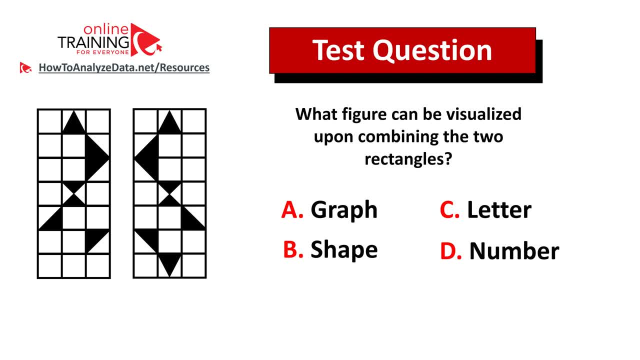 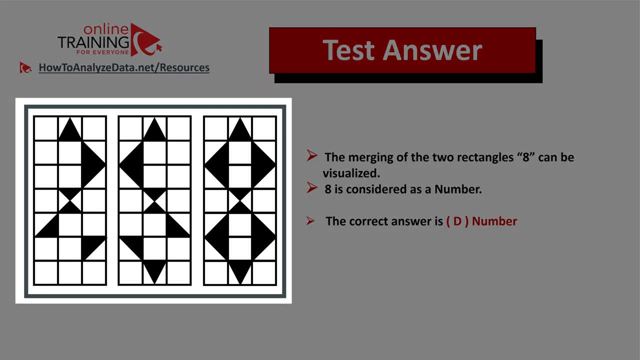 Did you figure out the solution? Let's continue to see how we can get to the correct answer together. Let me explain to you how you can come up with the solution on your own. Upon merging of two rectangles, you can see that 8 can be visualized. 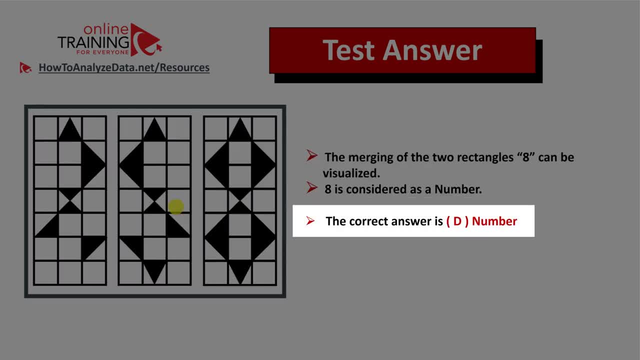 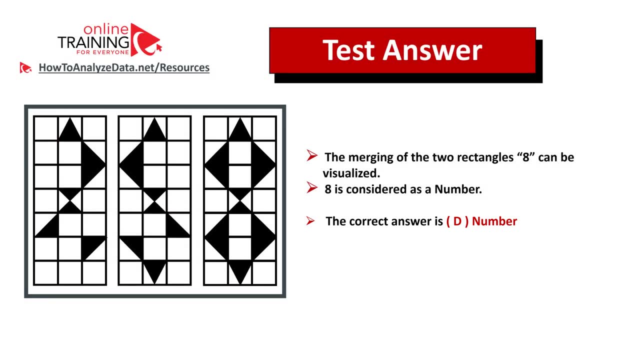 And 8 is the number, So the correct answer is choice D number. Hopefully you've nailed this question and now know how to answer similar problems on the test. And now here's the question for you to try: Which of the following does not belong to the group? 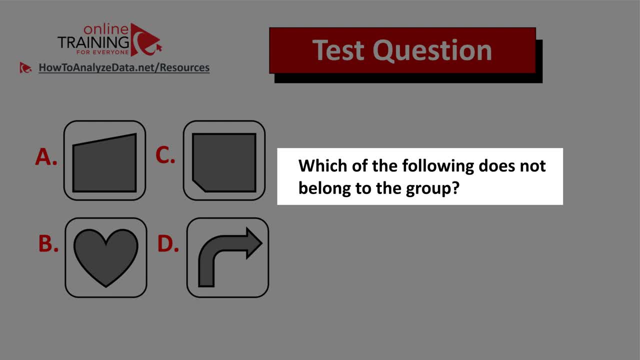 I have full confidence that you can solve this challenge from the real test by yourself. You're presented with four different rounded squares. Each one has a shape inside Choices A, B, C and D. Do you see the answer? My tip for you: always look for patterns. 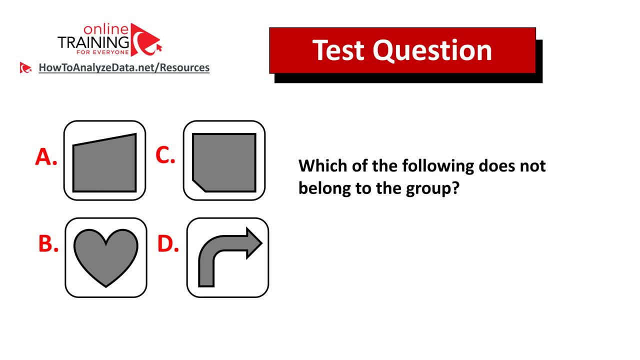 So which of the following does not belong to the group? Maybe give yourself 10 to 15 seconds to see if you can come up with the answer on your own, And if you have figured out the answer, please make sure to post it in the comment section of this video. 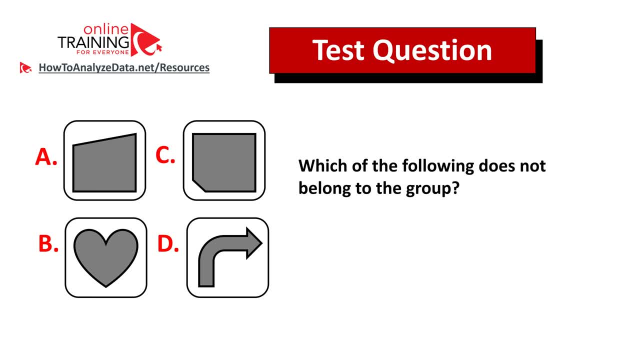 so I can give you my feedback. I'm also planning to post a detailed answer in my future videos, So make sure to subscribe and review my latest videos on the topic to learn about the answer to this and other assessment test questions. Thanks for participating. 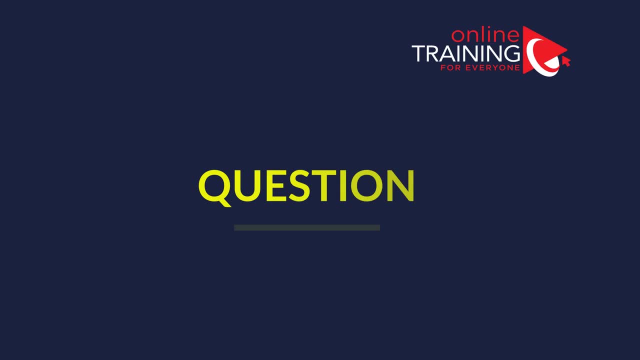 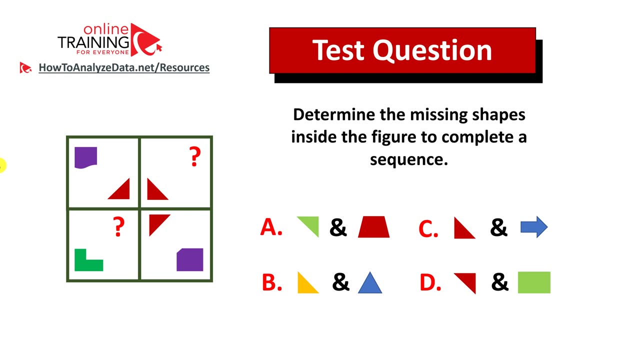 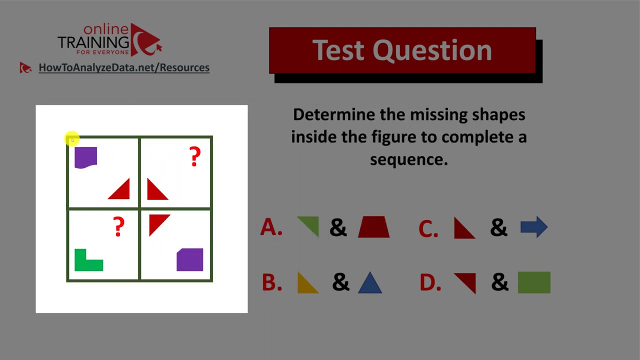 and good luck solving this challenge. Let's look at the interesting question which tests your pattern recognition skills. Let's look at the missing shapes inside the figure to complete the sequence And you're presented with 2x2 figure. It has two missing shapes. 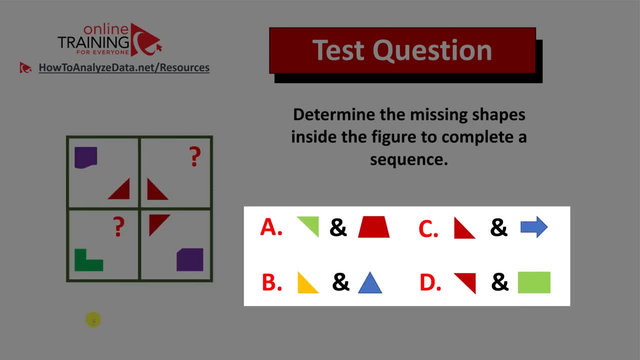 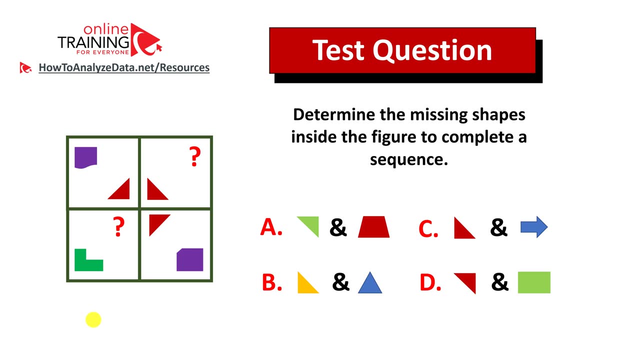 And you have four possible choices: A, B, C and D. Do you see the answer? Now might be a good time to pause this video and give yourself 10 to 20 seconds to see if you can come up with the solution on your own. 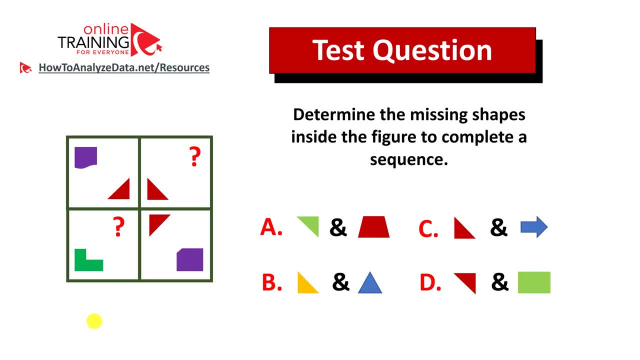 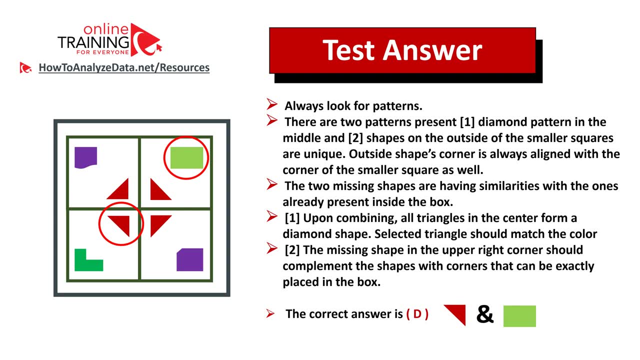 Did you figure out the solution? Let's continue to see how we can solve this challenge together. As usual, to solve these types of problems on the test, you need to look for patterns, And there are two patterns here presented. Number one is the diamond pattern in the middle. 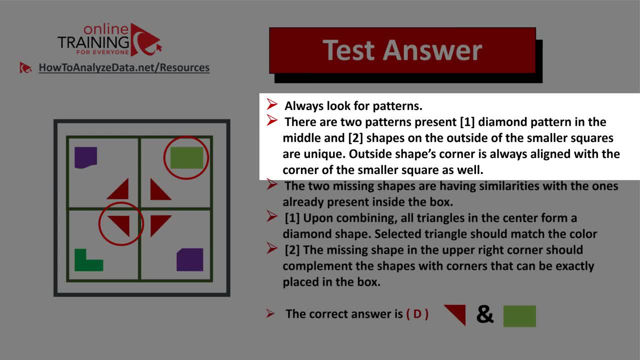 And number two is the pattern of shapes on the outside of the smaller squares, which are unique. Outside shapes, corners are always aligned with the corner of the smaller square as well. The two missing shapes also have similarities with other shapes present in the box Upon combining all triangles in the center. 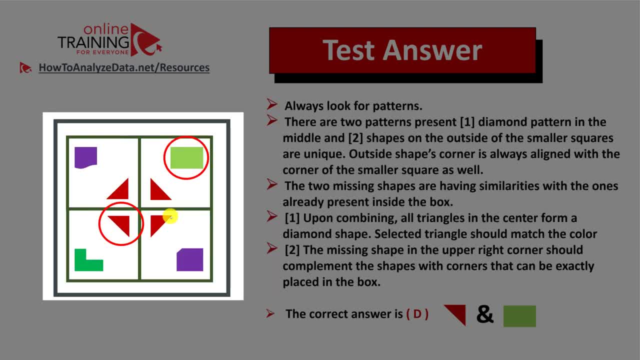 form a diamond shape. Let's look at each one of these two patterns in more details. You should look for the triangle which matches the color And, upon combining it, should build a diamond. For pattern two: the missing shape in the upper right corner. 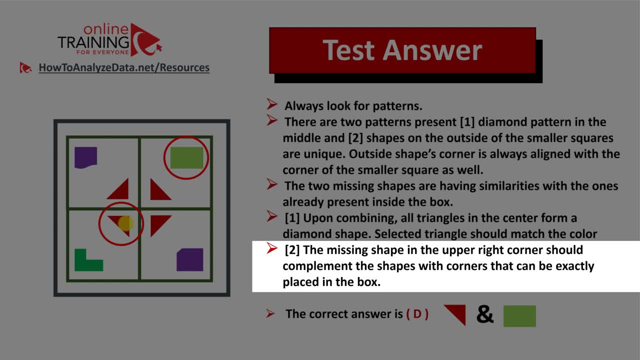 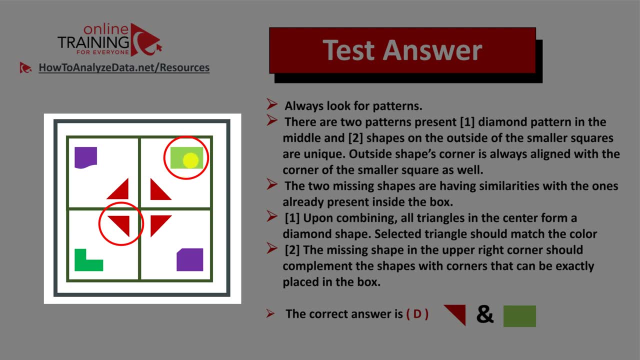 should complement the shapes with the corners that can be exactly placed in the box. In this case, we selected green rectangle. You also notice that there is a pattern of green color on the opposite side of the squares, Same as the purple colors on the opposite sides of other squares. 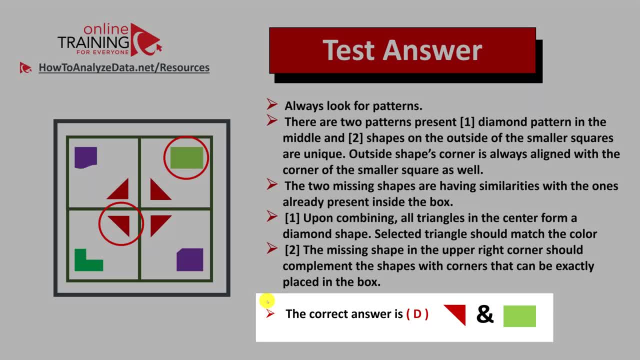 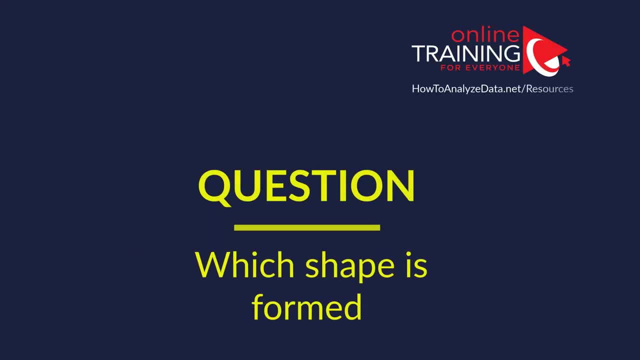 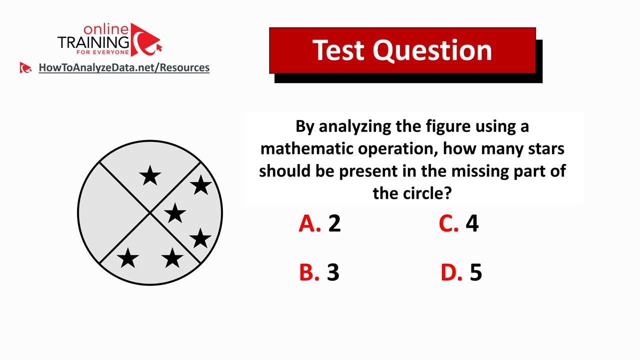 So the correct answer here is choice D. Hopefully you've nailed this question and now know how to answer similar questions in the test. Let's look at the tricky question which tests your knowledge of reasoning as well as the math skills. Here is the question. 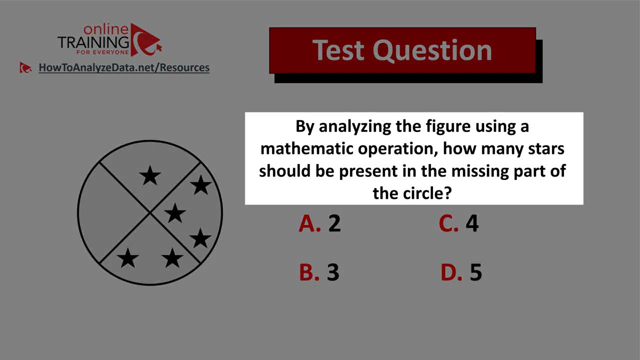 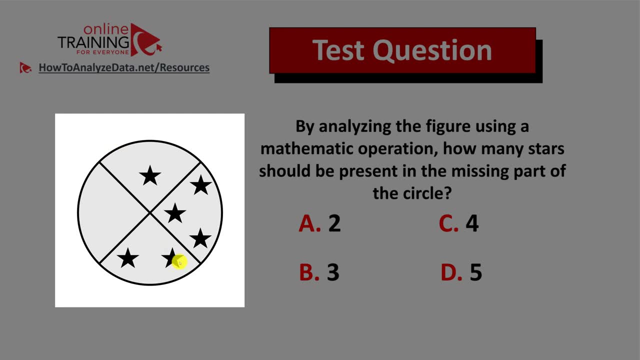 By analyzing the figure using a mathematical operation, how many stars should be present in the missing part of the circle? And you have a circle broken down into four equal parts. Three parts of the circle already have stars And they have one, two and then three stars. 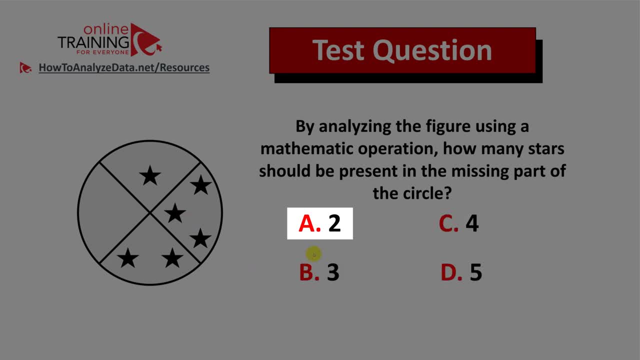 And you have four different choices: Choice A two, Choice B three, Choice C four And choice D five. So can you determine how many stars should the blank part of the circle have? Give yourself 10 to 20 seconds. 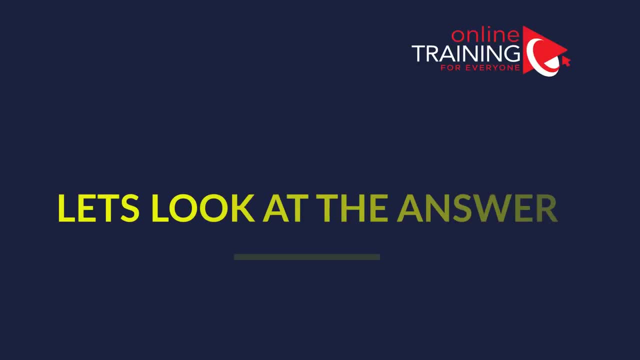 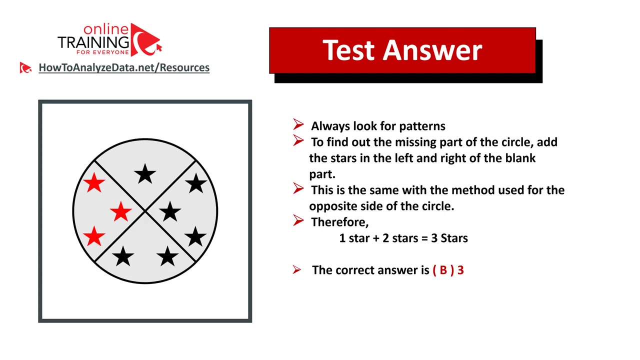 to see if you can come up with the answer on your own. Did you figure out the answer? Let's continue to see if we can come up with the solution together, As usual, to answer any type of question, look for patterns, And here the pattern is symmetricity. 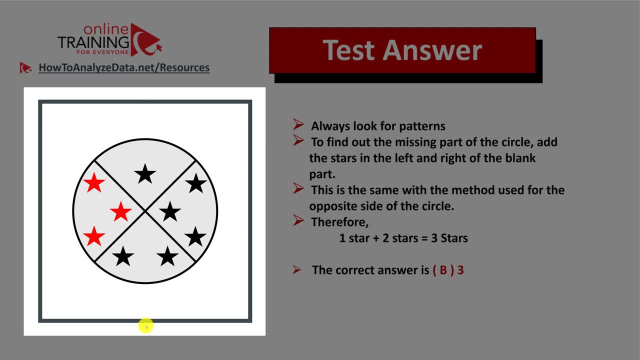 So if you draw the line in the middle of the circle from top to bottom, you will see that you need to come up with the answer that would be symmetrical. There are multiple ways to solve this challenge and we got a hint: that we should use mathematical operation. 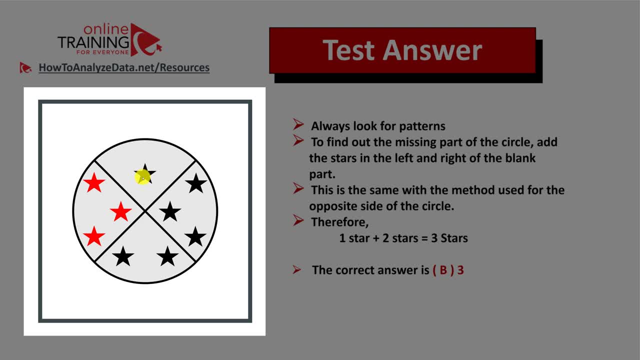 We take the star from the left of the blank part of the square and add number of stars from the right part of the blank square And we get one plus two, which is equal three. You can also use subtraction to come up with the answer. 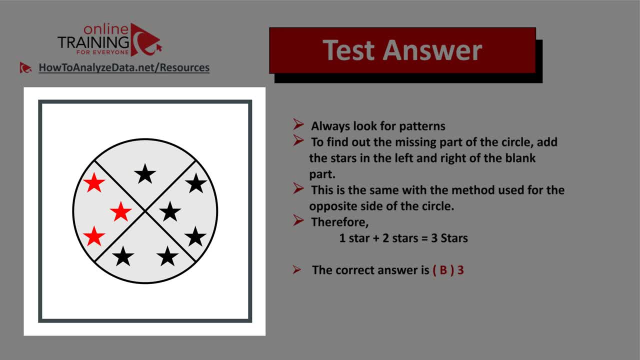 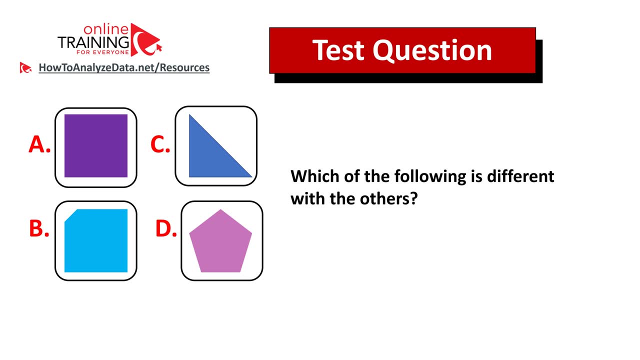 Can you figure out how to use subtraction to get to the similar answer? If you figure out the subtraction answer, please make sure to post it in the comment section of this video. And here is the question from the real test you can try to solve on your own. 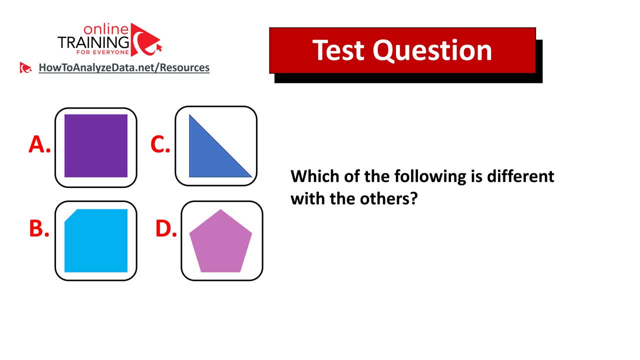 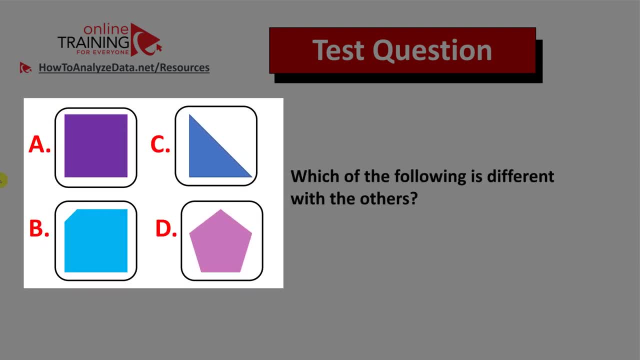 I have full confidence that you can really solve this challenge. Which of the following is different from the others, And you present it with four different shapes: Choice A- square, Choice B- different square, Choice C- triangle And choice D- pentagon. 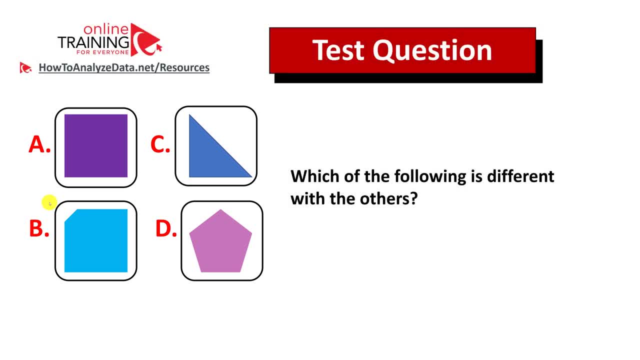 So which of the following is different from the others? Give yourself 10 to 15 seconds to see if you can solve this challenge on your own. If you figured out the answer, please make sure to post it in the comment section of this video. 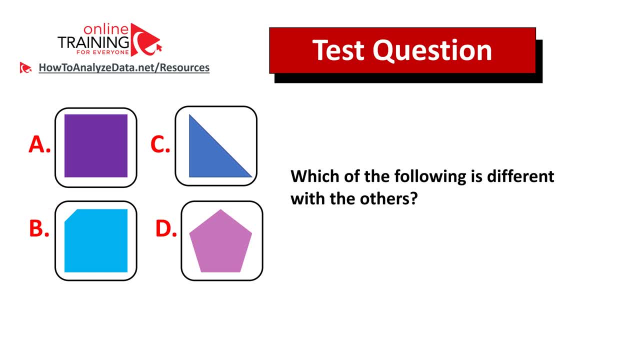 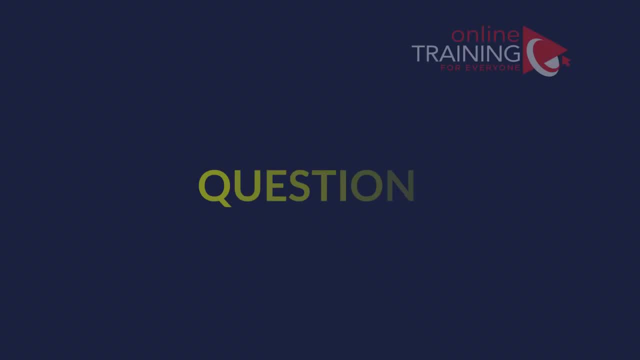 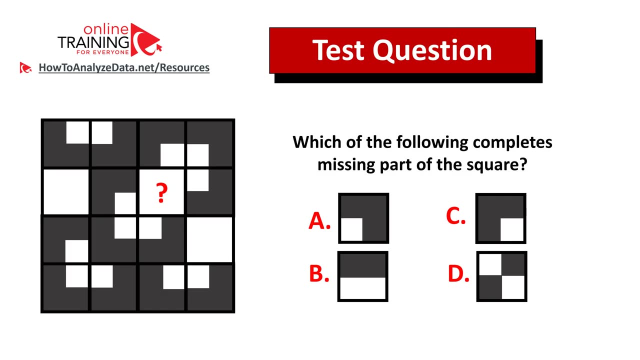 and make sure to include your rationale and how you solved it. This would allow me to give you feedback if your answer is correct. Thanks for participating and good luck solving this challenge. Let me share with you a tricky question which tests your pattern recognition and visual reasoning skills. 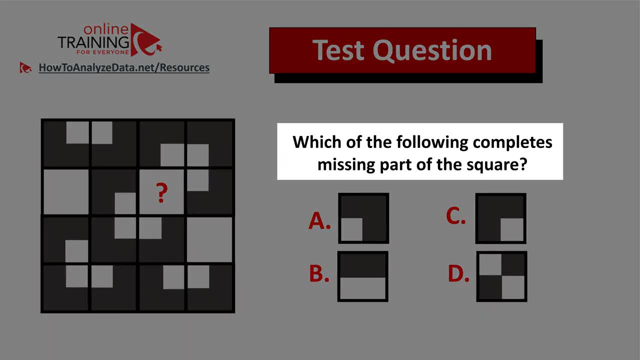 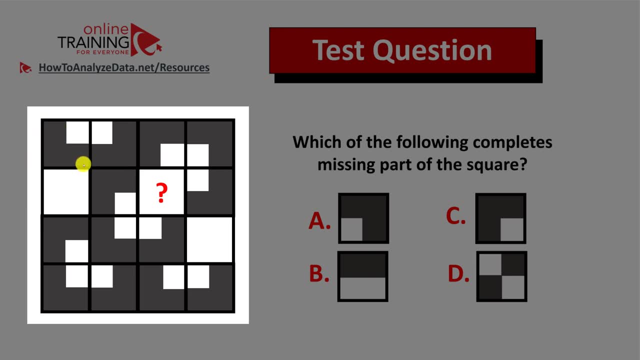 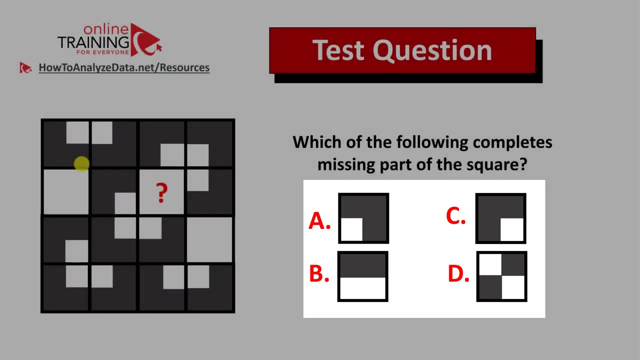 Which of the following completes missing parts of the square And you present it with the 4x4 square, which contains different smaller squares inside And four possible choices: Choice A, B, C and D. Do you recognize the pattern? 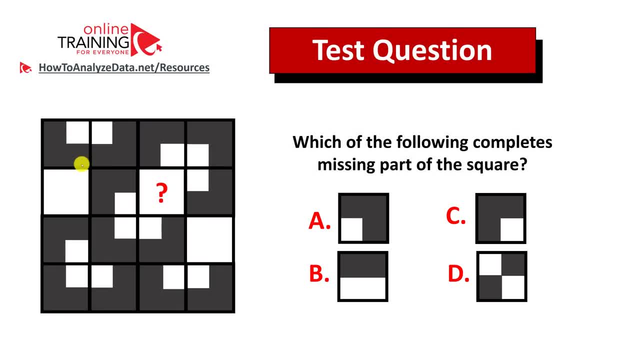 Now might be a good time to pause this video and give yourself 10 to 20 seconds to see if you can come up with the answer. Did you figure out the answer? Let's continue to see how we can solve this challenge together. Interesting question, isn't it? 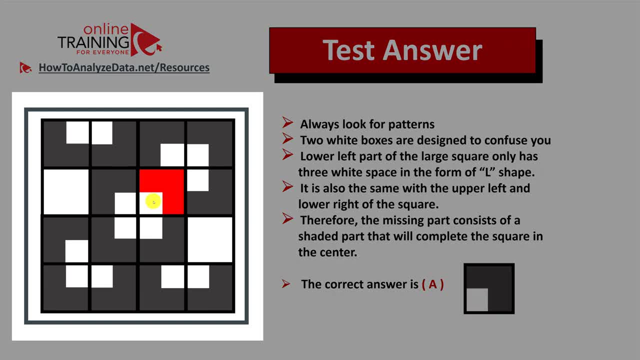 But as usual, look for patterns. If you look closely you will see that the middle box, right in the center of the larger square, is symmetrical. So the L shape at the bottom and in another shape in the upper right corner, they represent symmetricity. 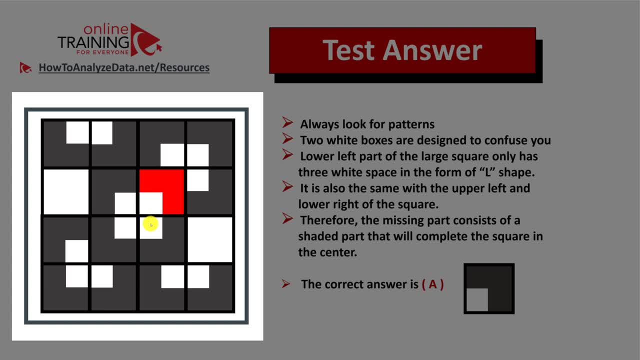 for this middle square, which consists of the four small squares. Couple important considerations when answering this question. Two white boxes designed to confuse you. Lower left part of the larger square only has three white spaces in the form of L shape. Similar symmetrical pattern. 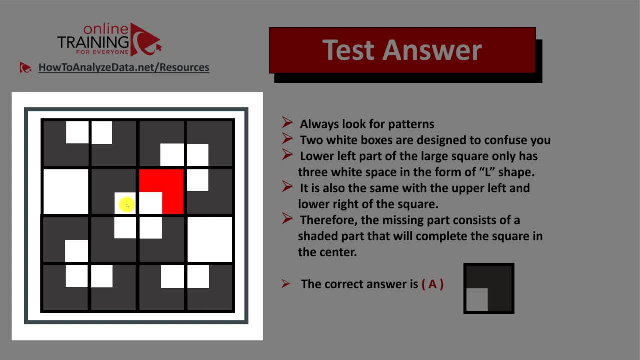 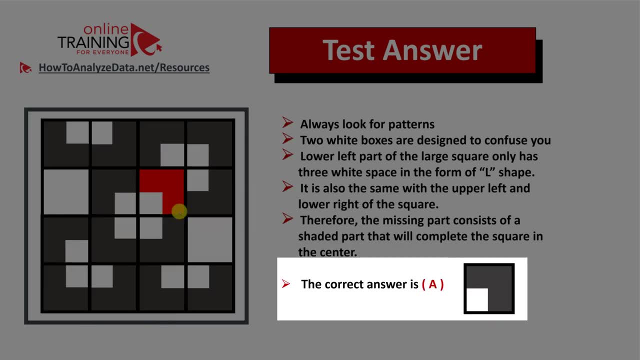 follows in the upper right corner. This is why the missing part consists of the shaded part, which completes the square in the center. So the correct answer here is choice A. Hopefully you've nailed this question and now know how to answer similar problems on the test. 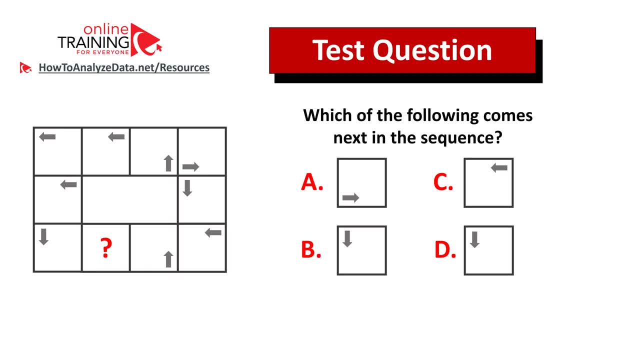 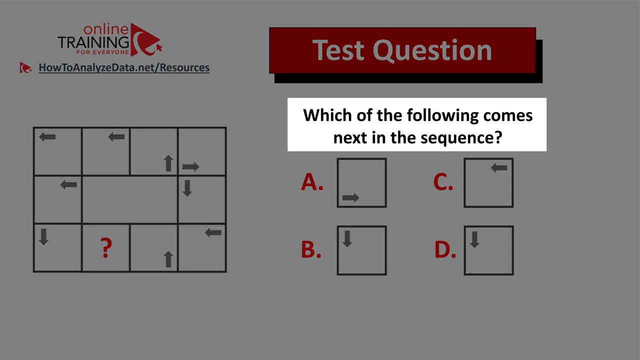 Let me share with you a tricky question which tests your pattern recognition as well as logical reasoning skills. Which of the following comes next in the sequence? and you are presented with rectangle Which has multiple squares and one of the squares is missing. it has a question mark inside. 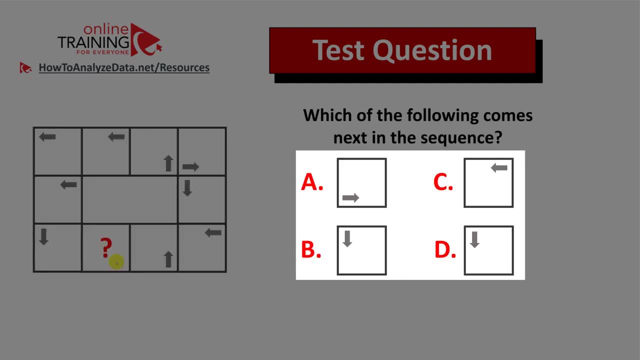 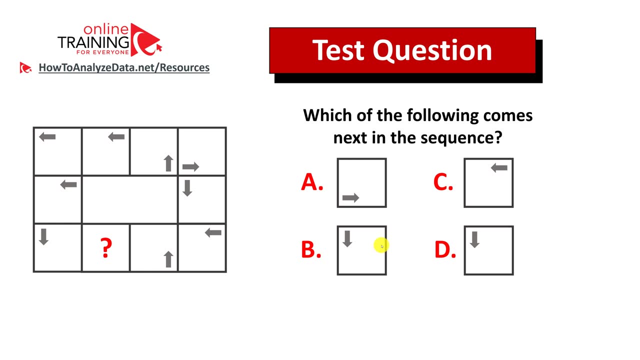 and you have four different choices: A, B, C and D. Take a close look to see if you can come up with the answer Now. may it be a good time to pause this video to see if you can come up with the solution on your own. 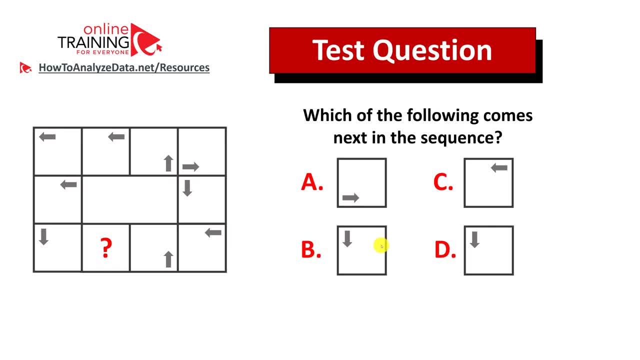 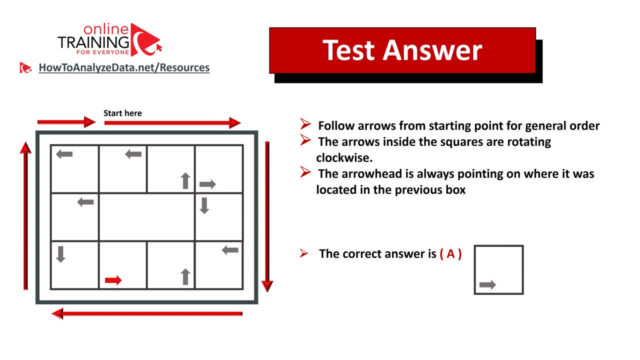 Did you figure out the answer? Let's continue to see how we can get to the correct solution together. There are a couple tricky parts about this question. Number one is the general flow of squares And then there is a sequence of arrows inside the squares. 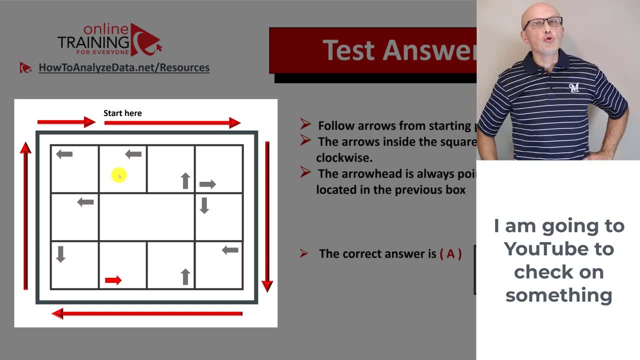 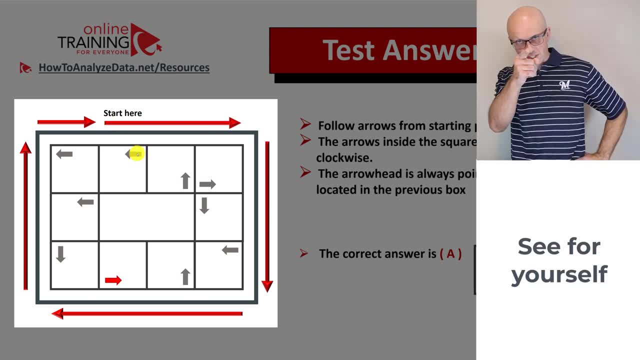 For example, we're starting the flow right here, not in the corner, It's kind of in the middle of the upper row, And then you need to follow the red arrows for the general order, The arrows inside the squares rotating clockwise, And what you can see is the arrowhead.